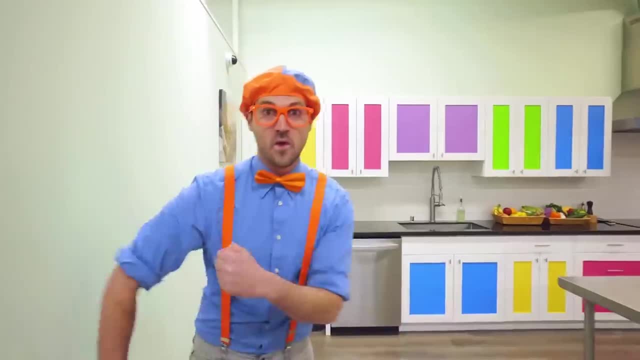 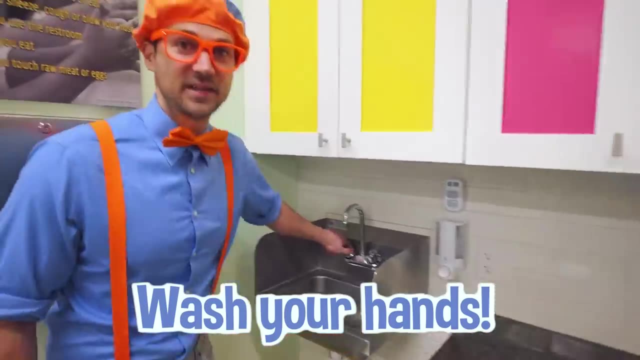 Whoa, come on. Okay, the very first thing that I need to do when we enter a kitchen is wash our hands. Okay, I'm going to turn on the hot water And then I'm going to. I'm going to rinse them. 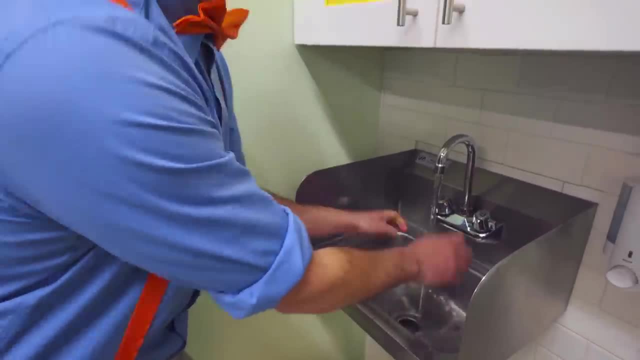 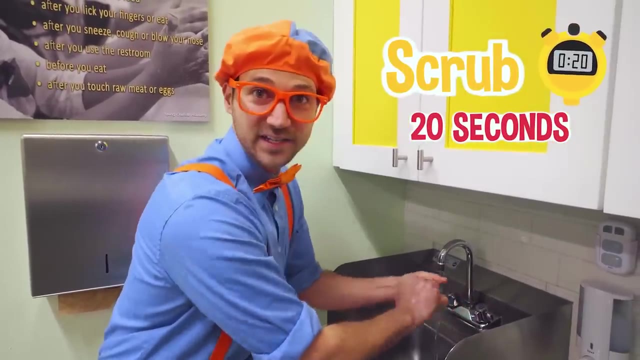 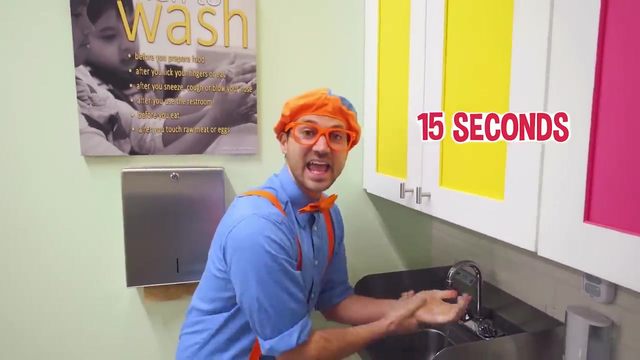 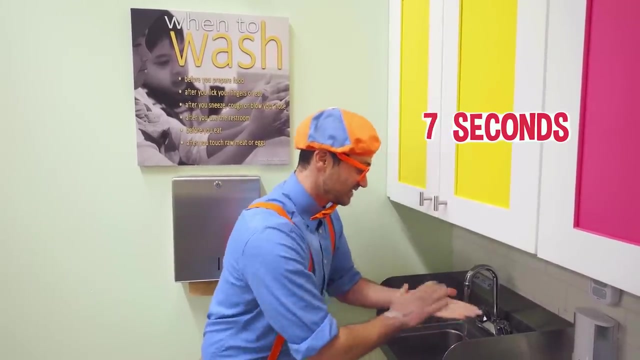 Okay, get them nice and moist. And then we need some soap, Okay, and we need to scrub for 20 seconds. And one way to do this is to sing the ABCs Ready: A, B, C, D, E, F, G, H, I, J, K, L, M, N, O, P, Q, R, S, T, U, V, W, X, Y and Z. 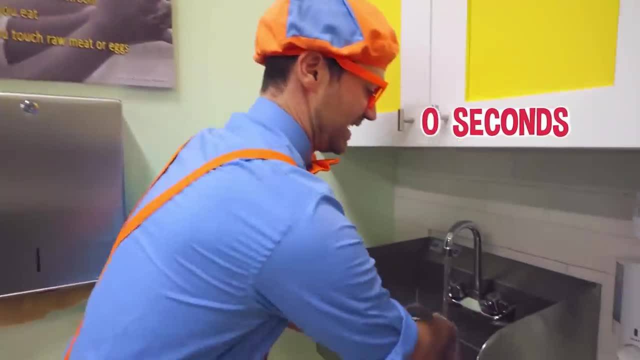 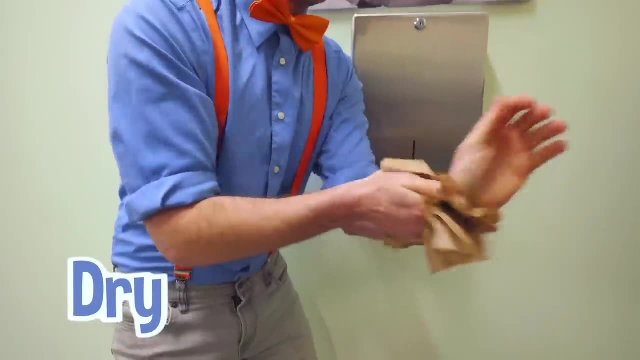 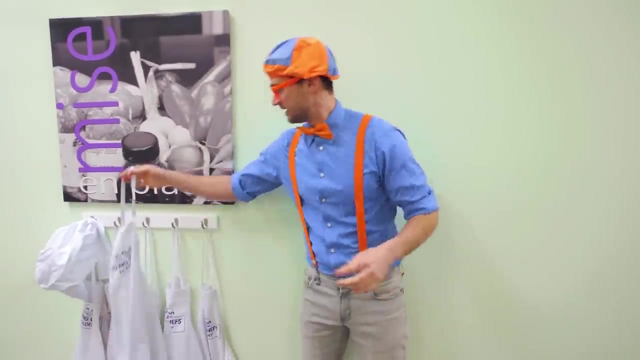 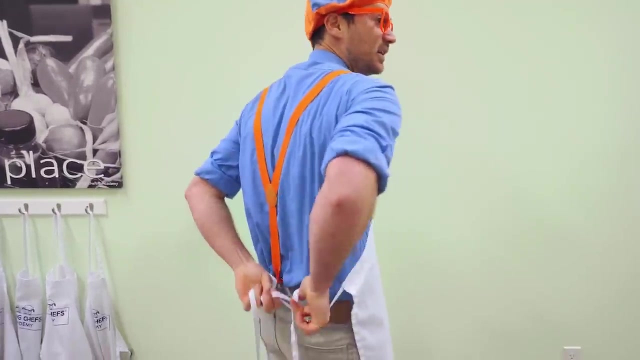 Okay, now we're going to rinse off our hands. Get them nice and dry Now. once our hands are dry, clean, now we can put on an apron. Yeah, an apron is used. so then, clothes not get dirty when you're cooking. 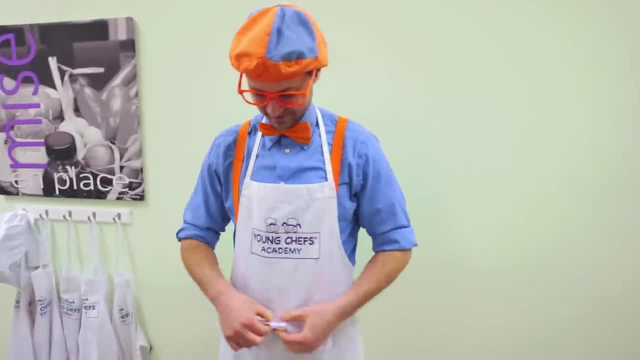 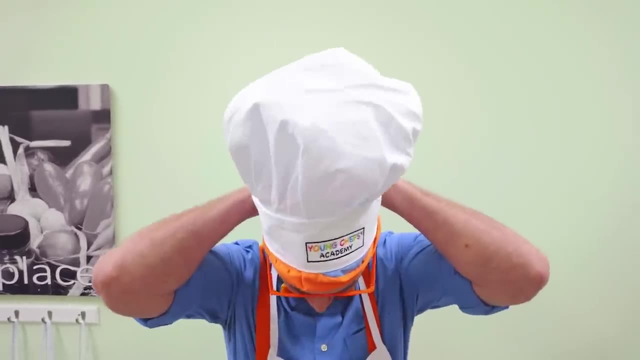 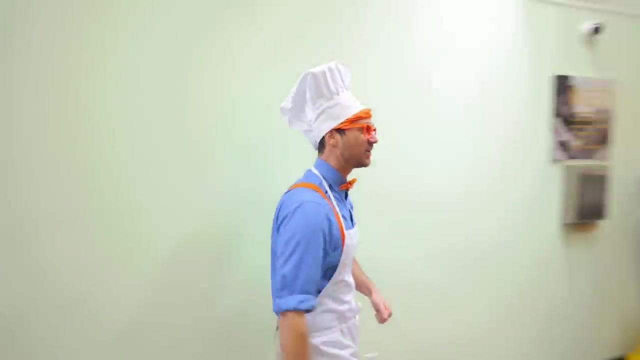 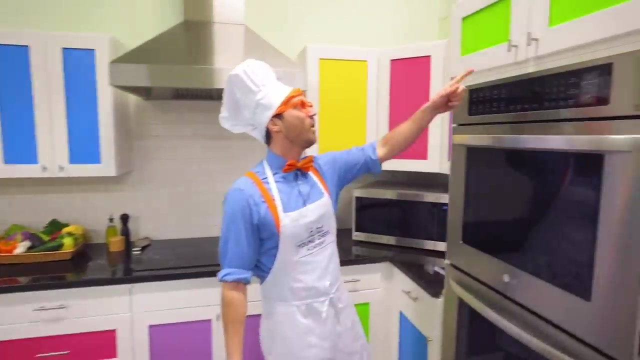 With some food, All right, And can't forget my young chef's academy chef's hat. How do I look? All right, Check it out. This kitchen is so colorful. Do you see all these cabinets? Yeah, Whoa, These, yeah, are the color green. 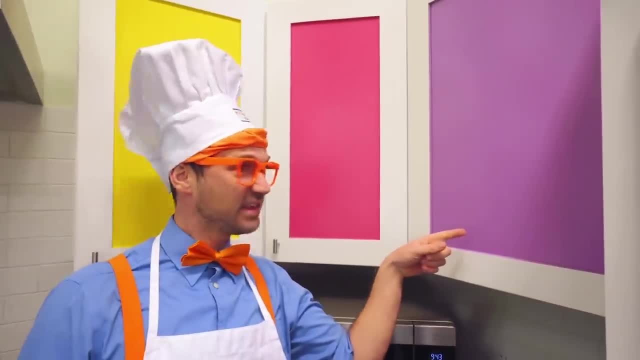 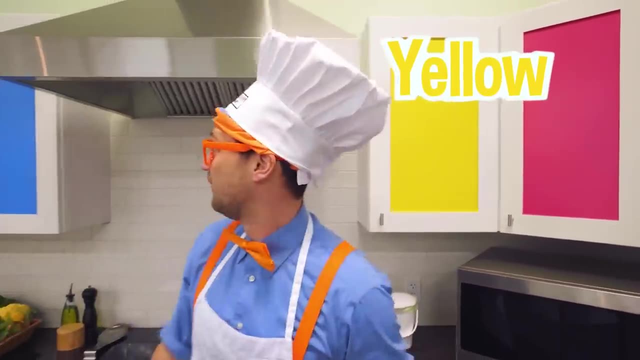 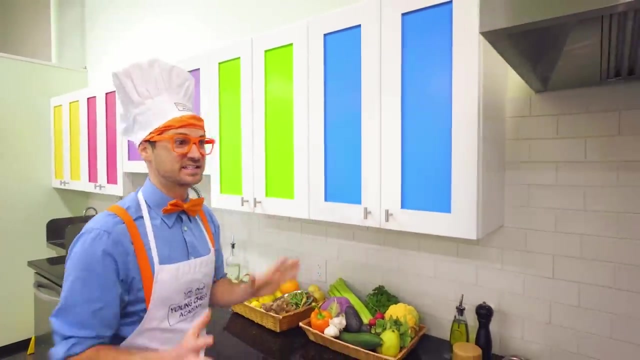 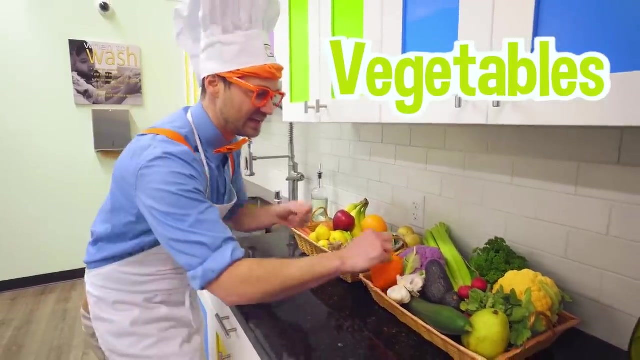 Ooh, this over here. yeah, that cabinet is purple, pink, yellow and blue. Whoa, I bet there's a lot of cool things in these cabinets. Whoa, Look at this, Some yummy vegetables. Hey, you know what kind of vegetable this is? 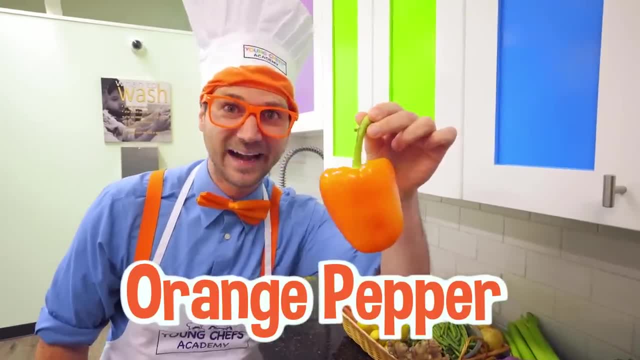 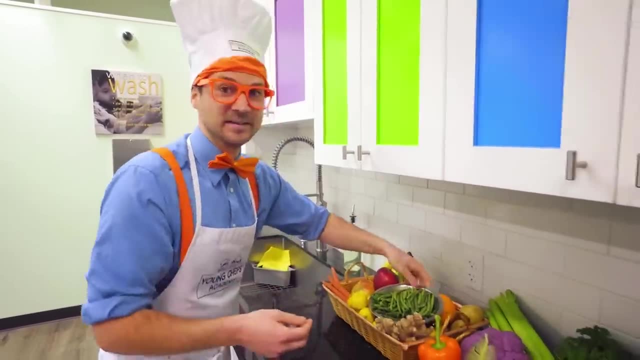 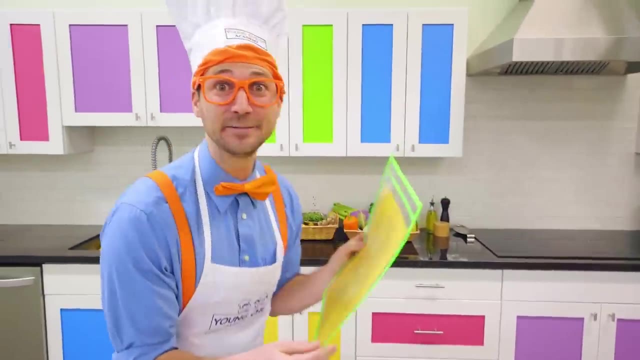 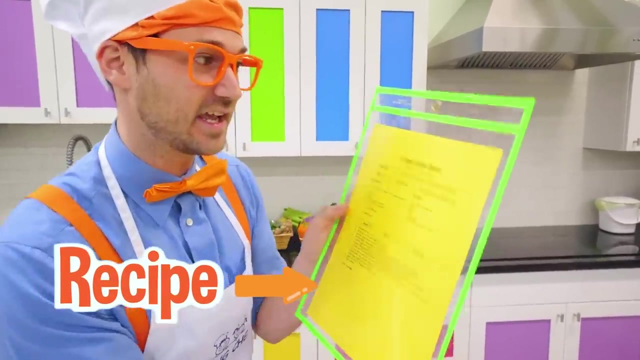 Yeah, This is an orange pepper. Look at these. Yeah, some green beans. I sure do love vegetables. All right, I'm so excited. Whoa, I am so excited. This is going to be tasty. I am looking at the recipe of what we're going to be making today. 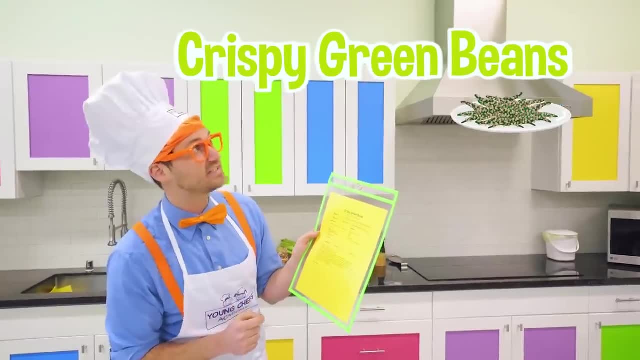 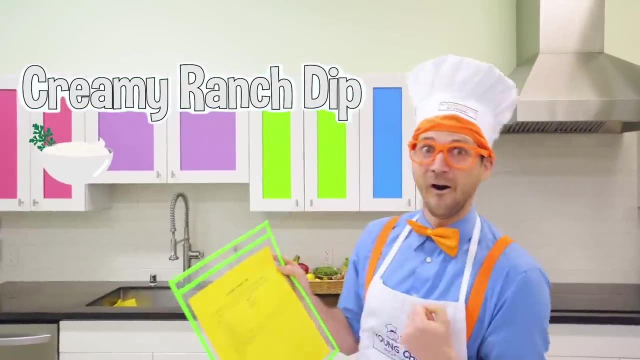 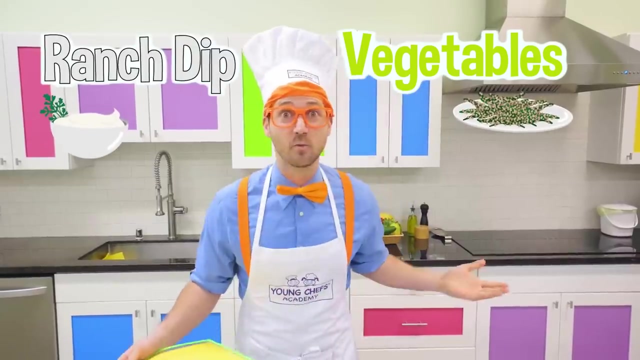 Looks like we're going to be making crispy green beans- Whoa, Those look tasty- and creamy ranch dip- Oh, this is going to be so yummy and healthy. I love vegetables and I love ranch dip. I wonder if we're going to be able to dip the green beans into the ranch dip. 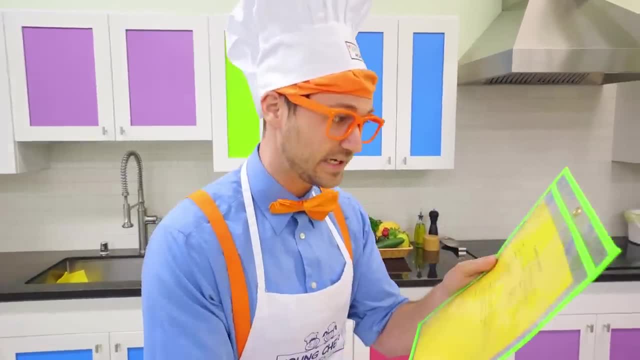 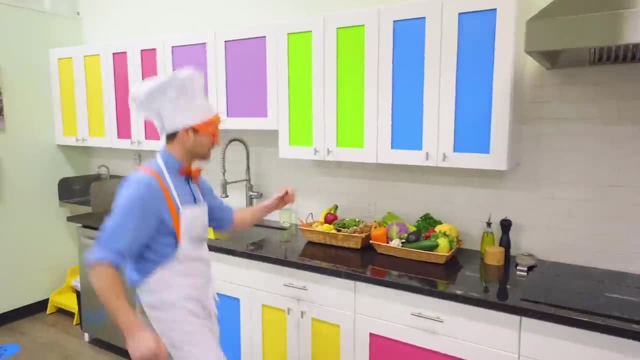 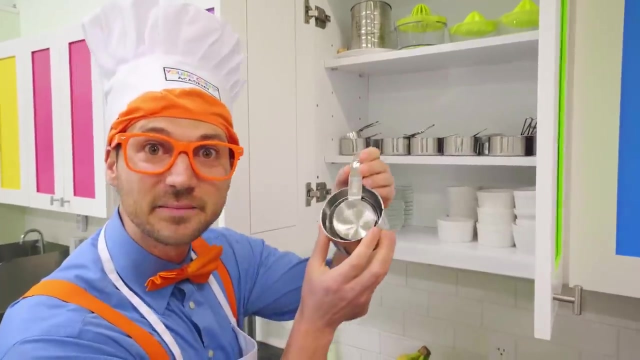 Yeah, Okay. So it seems like we need a lot of tools and a lot of ingredients, So let's get to it. All right, Let's see what's in here that we need. Okay, Looks like we need some measuring cups. 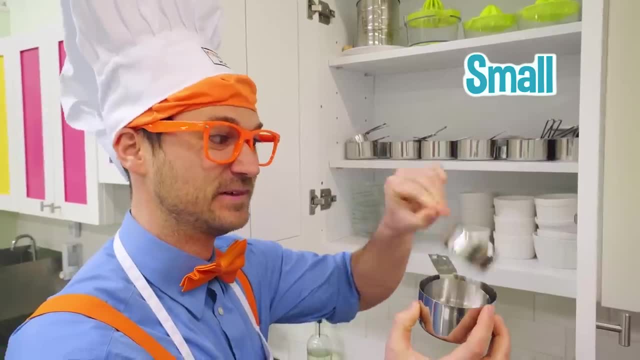 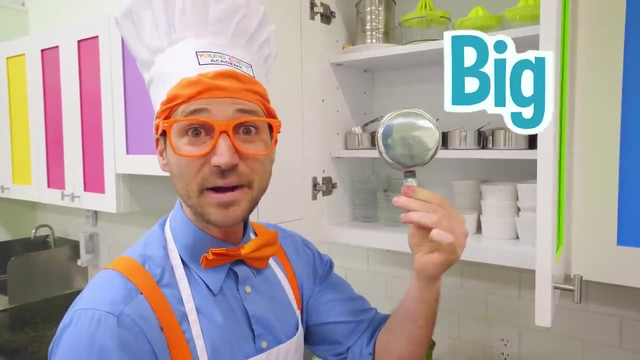 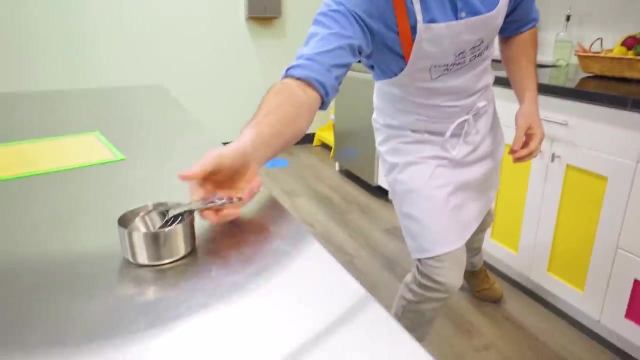 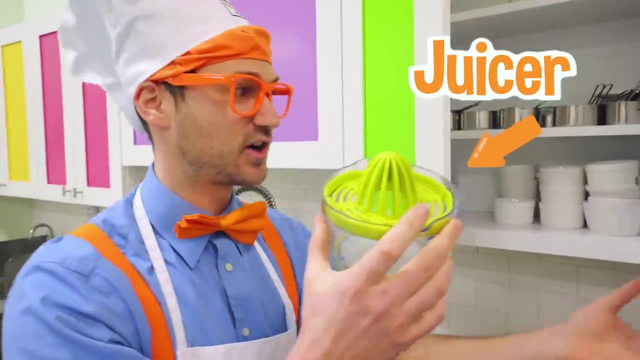 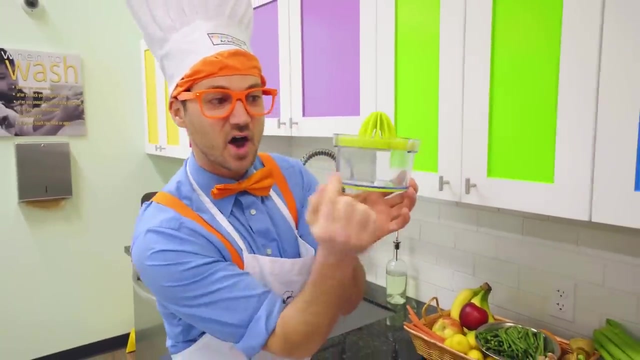 Oh, a small one, A medium-sized one, Another medium-sized one And a big one. Okay, Put those right back here. Perfect. Then we need Whoa, A juicer. This is where you can put a lemon or an orange or a lime, squeeze it on top and then all. 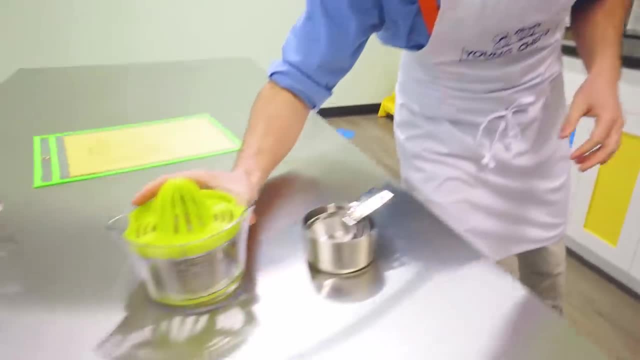 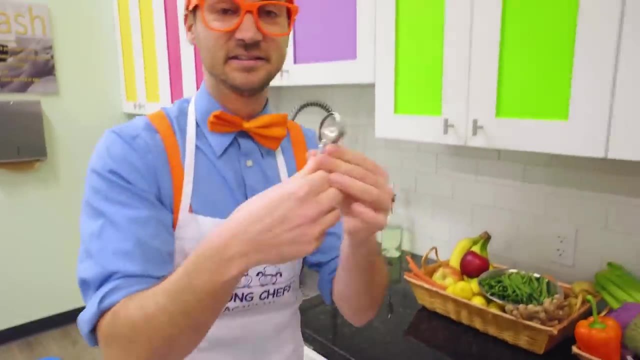 the juice comes out the bottom. Okay, We'll set that down right there. All righty, Let's see what's in here. Hmm, Oh, We definitely need some measuring spoons. Whoa, Yeah, Same thing, Just like the measuring cups. 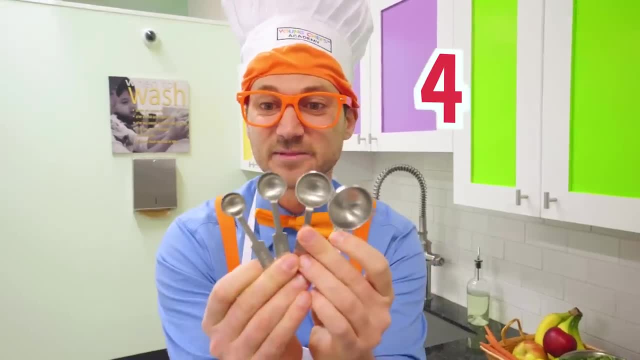 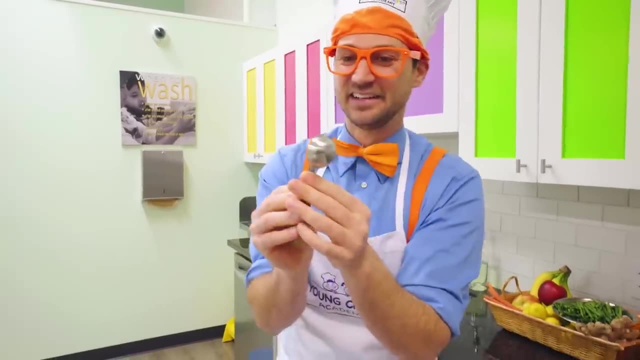 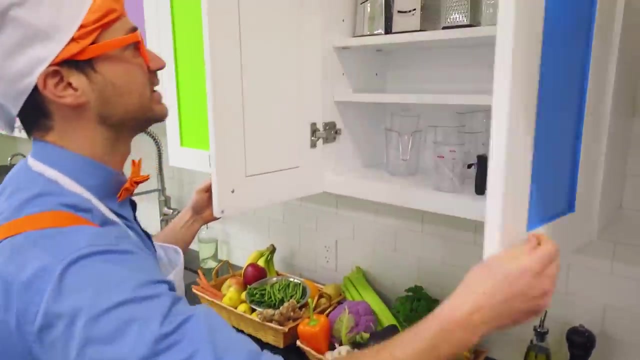 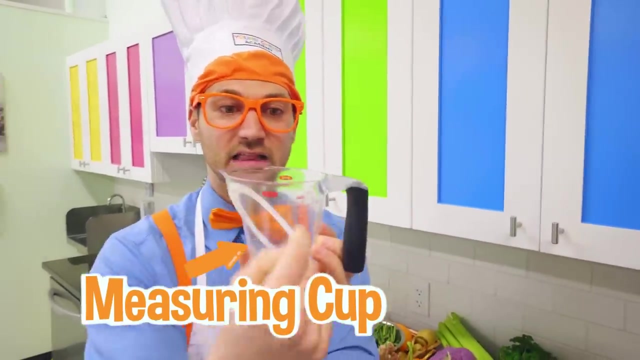 Measuring spoons of four different sizes, From small to medium to medium to large. Okay, Put them right in there, Perfect. Okay, Let's see How about? Oh Wow, A measuring cup. This is what you put: liquids, and you could do solids, but this is primarily for liquids. 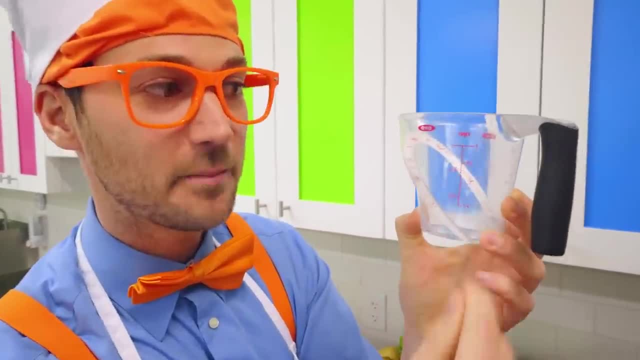 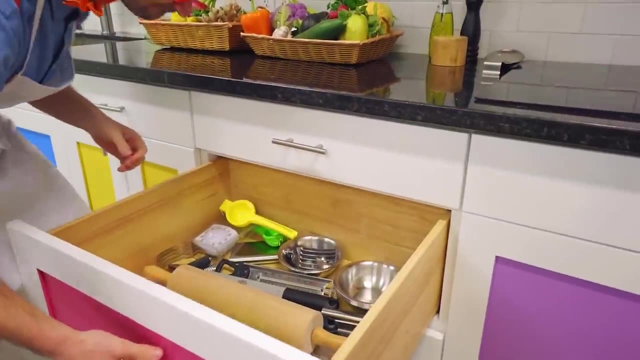 And this is what you measure, to see how much you have. Okay, Put that down right there. Oh, Let's see. Is there anything in here? Hmm, There's a lot of cool things in here. Whoa, Look at this. 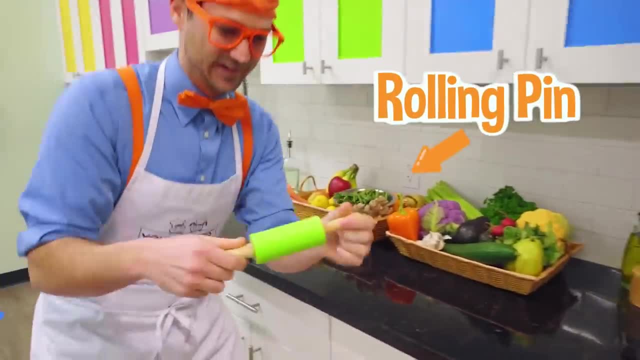 It's a rolling pin. Oh, So cute. This is a small rolling pin Whoa. And this is a big rolling pin Whoa. They're used to flatten things out, And this is a big rolling pin Whoa. 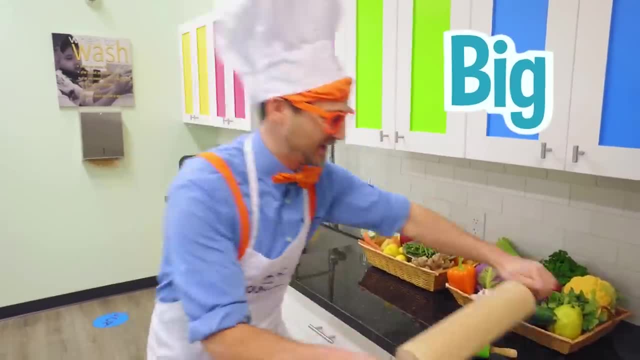 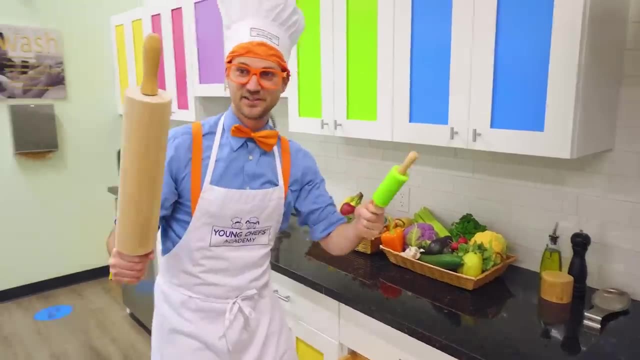 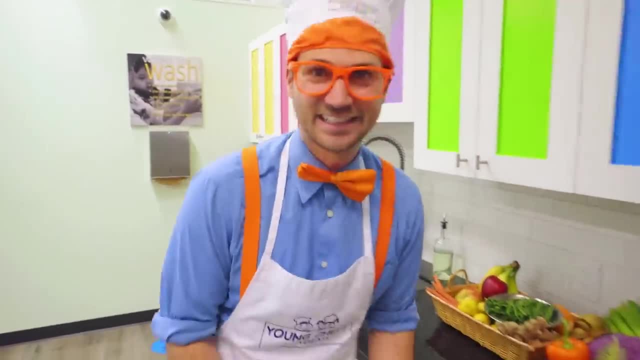 I don't think we need those today, but they're pretty cool because you can use them for drums. Okay, That's plain. Let's get to cooking. All right, Let's see Probably right in here. Oh yeah, Two ingredients that we need. 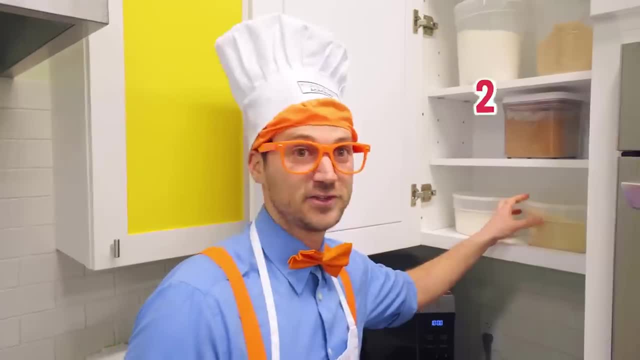 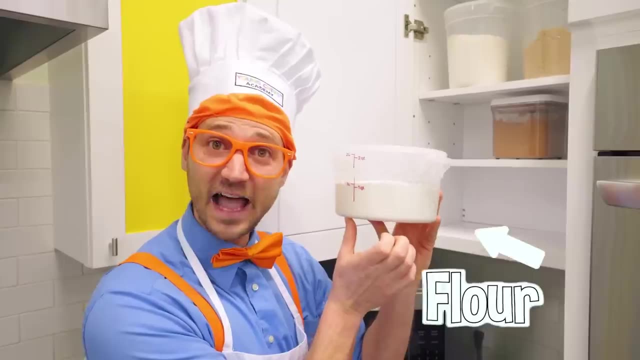 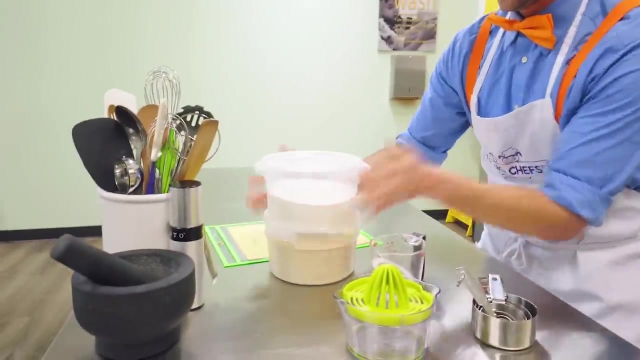 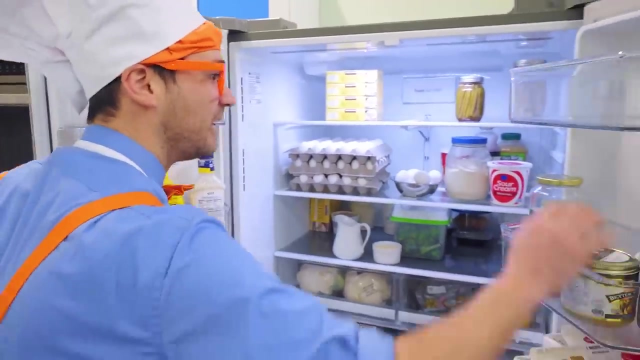 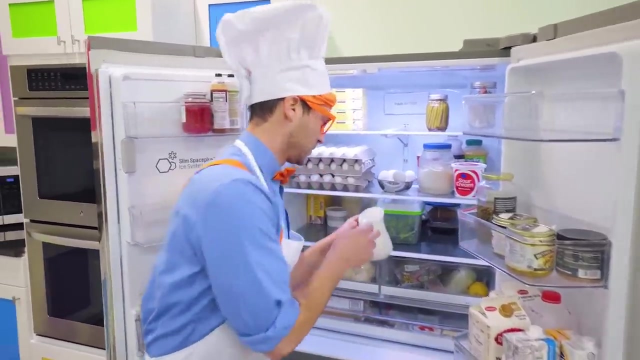 Breadcrumbs And flour: Perfect, Okay, We'll shut this. Oh, Cool, Awesome. So we have our ihnen. Okay, You want to try it? right, there we go. and let's see about some cold ingredients. whoa, look at this fridge. it's so organized, okay, looks like we have some. 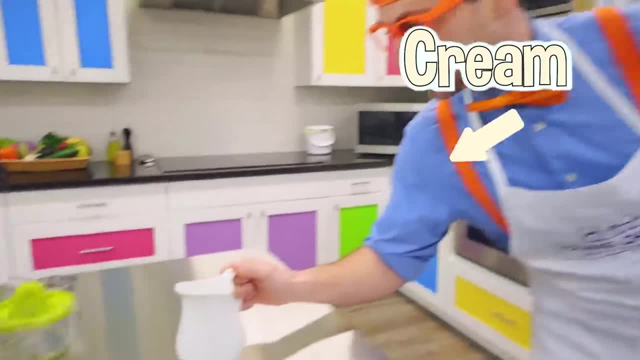 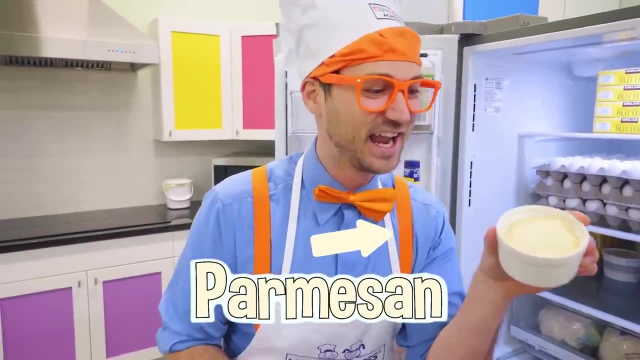 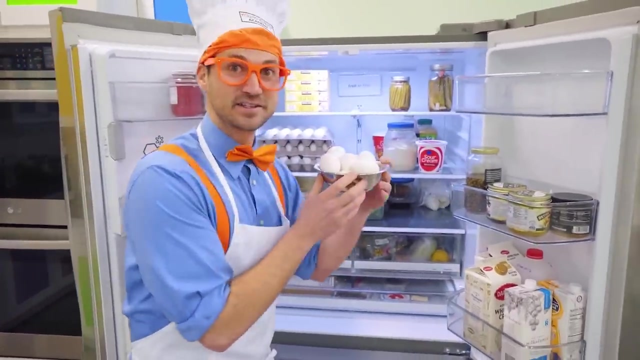 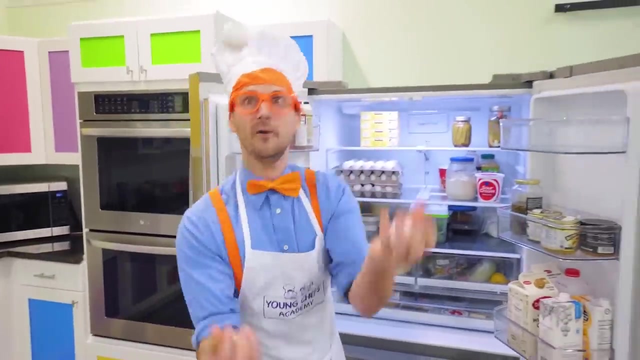 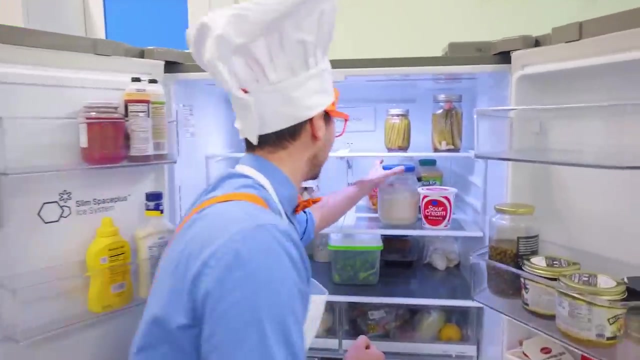 cream, probably for the ranch dip. we'll set that down right there. oh, some cheese, parmesan cheese- okay, put that down right there. and then we have some eggs- yeah, check this out. whoa, whoa. okay, put those down right there for later. probably shouldn't do that at home. and then we have some mayonnaise. 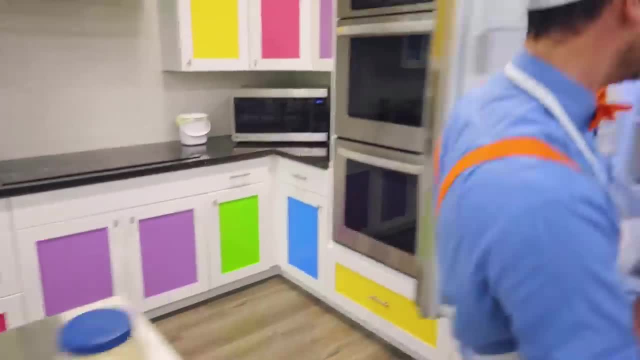 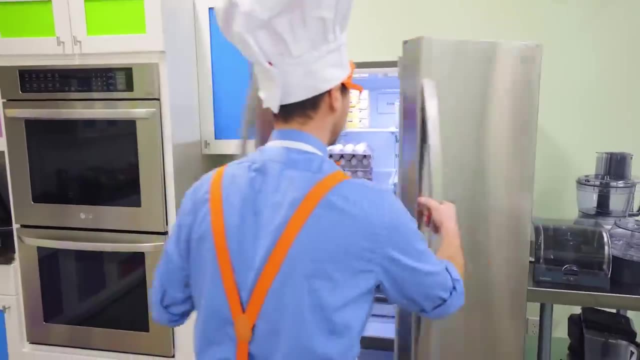 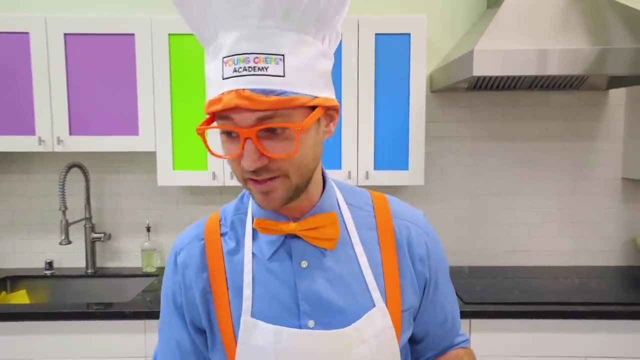 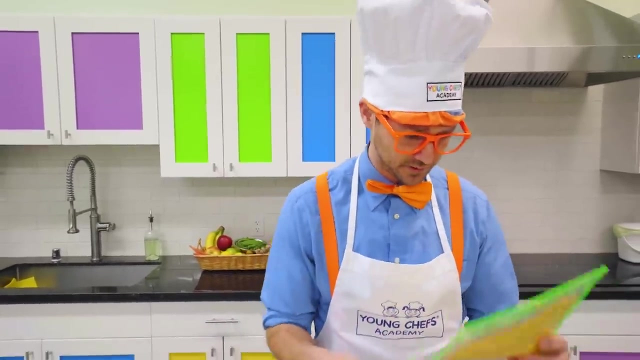 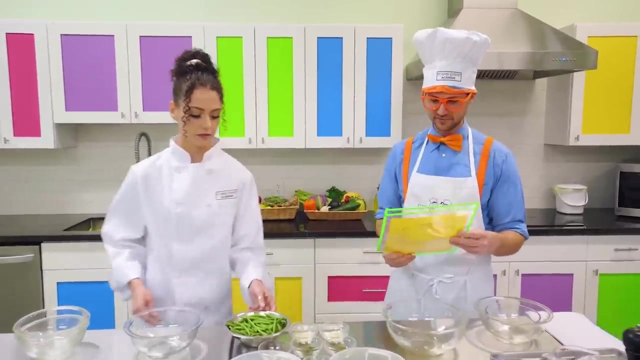 okay, put that down right here. and some sour cream: okay, put that down. and now I think we're ready. looks like we have most of the ingredients and tools, but this looks really hard. oh no, if only I had some help, we can put this together to make everything that we need perfect. 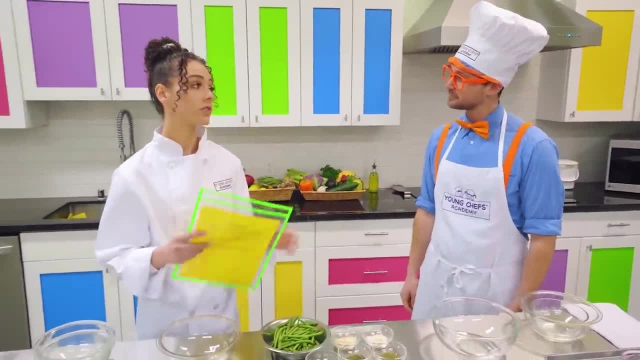 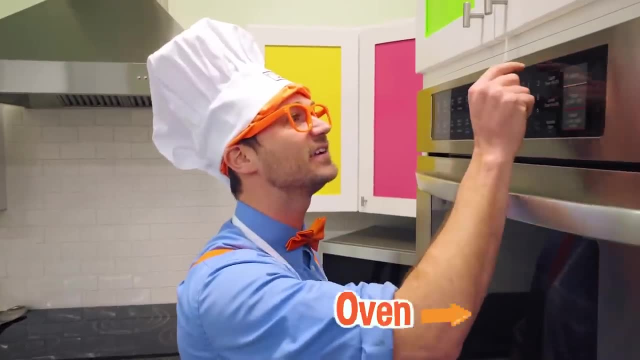 okay, here's the recipe. what do we do first? first, we're gonna want to preheat the oven to 425. okay, I know how to do that. okay, preheat the oven to 425. perfect, my job. good indeed. thank you all right. first, we're gonna want to do a. 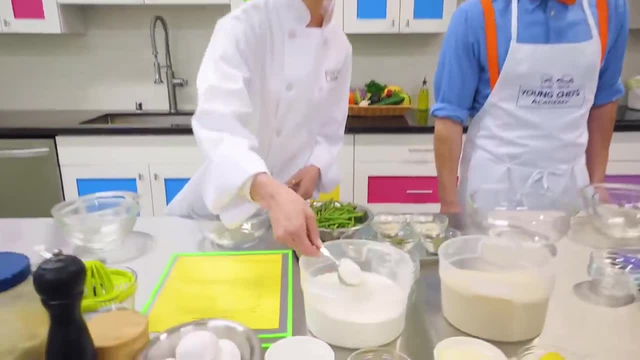 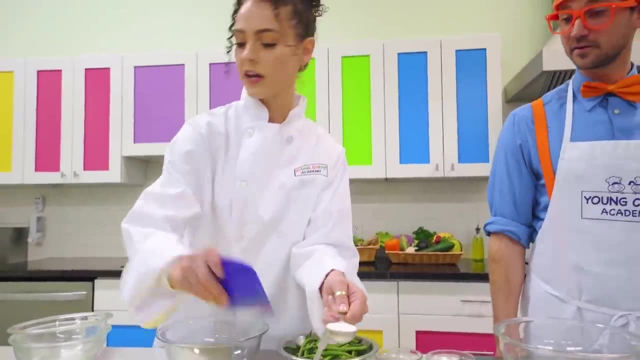 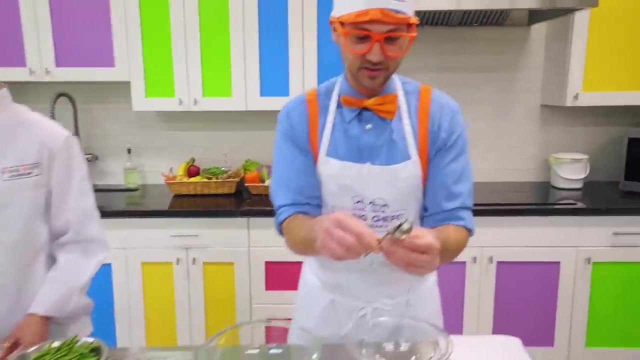 tablespoon of flour into our bowl. we're gonna want to make sure that we get a Tracy. she's starting at very lower true tablespoon, because that is not accurate. we're gonna scrape off the extra flour. so we're gonna scrape off the extra flour. Okay, can you do that? Sure, Okay, looks like we need some flour. Let's do a little scoop. 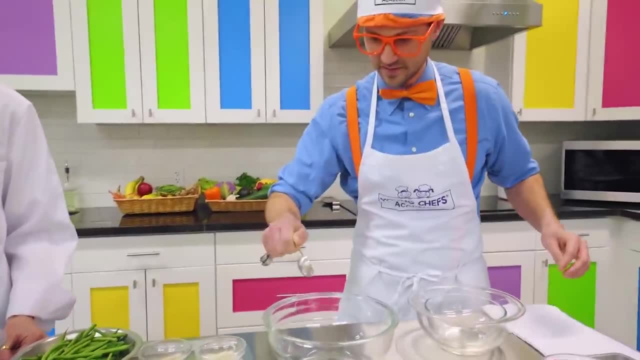 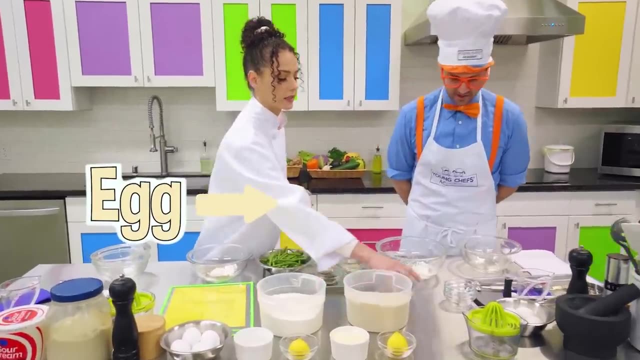 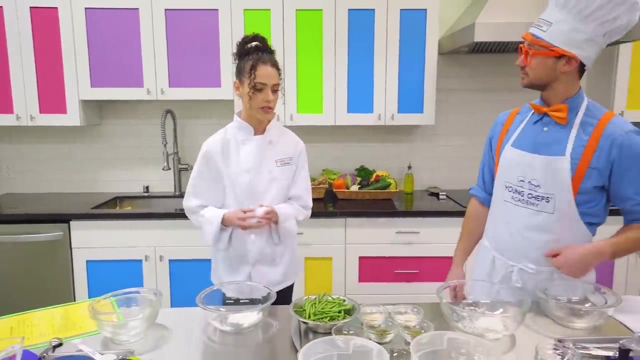 And there we go And perfect. Great job, Lippie. All right. next we're going to want to crack an egg. Okay. So at Young Chefs Academy we crack an egg using the table, not the edge of the counter, so that it doesn't get all over the floor and miss. Okay, You want to crack hard and use your 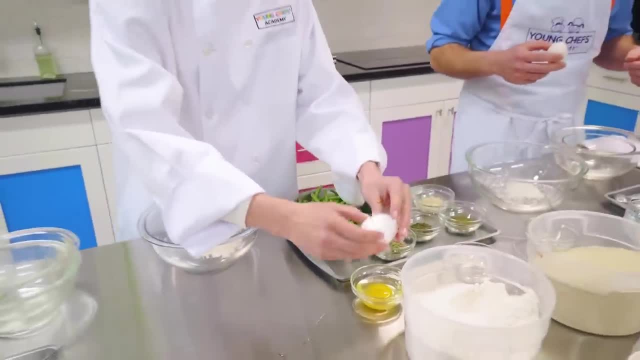 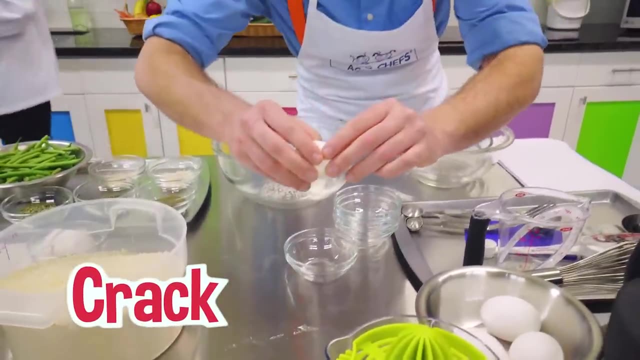 thumbs to break open the egg, just like that. Perfect. You don't want to put the shell in a separate bowl? Okay, here we go. Let's use the table. There we go. Great job, Lippie, Thank you. Next, we're going to want to wash our hands because we touched a raw egg. 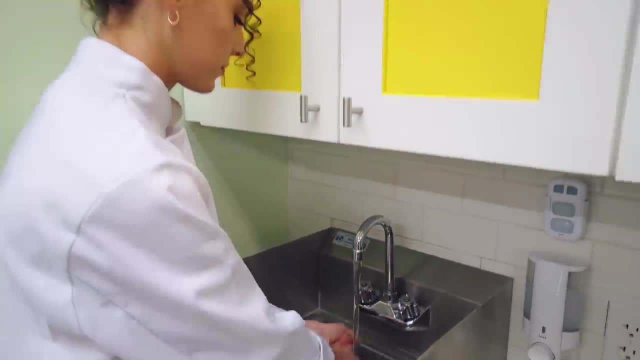 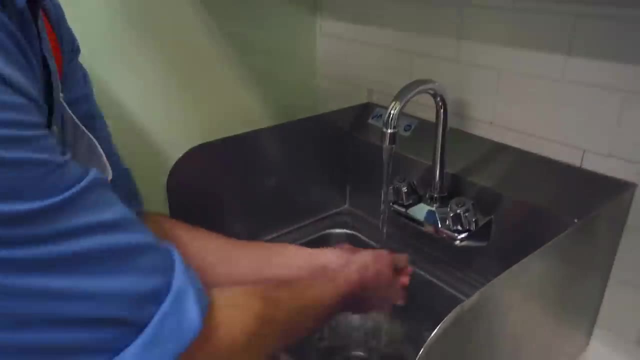 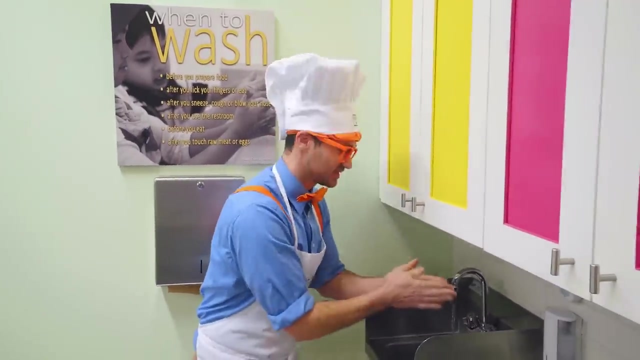 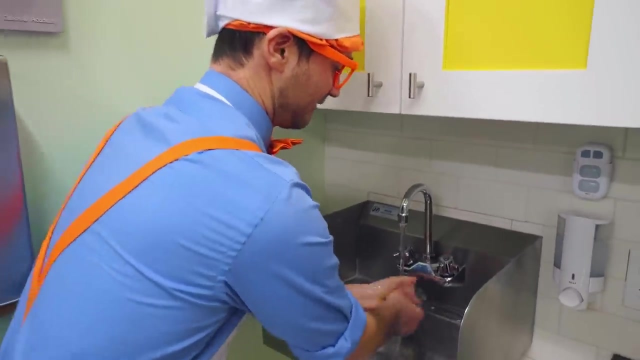 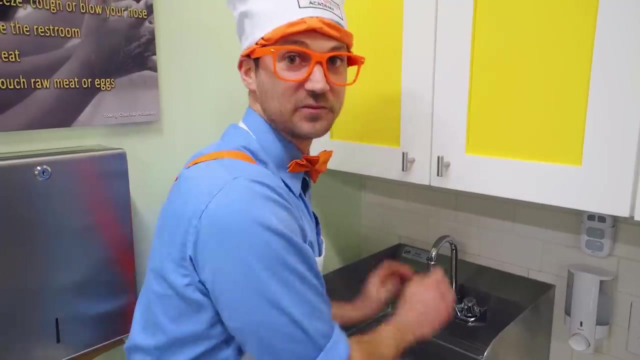 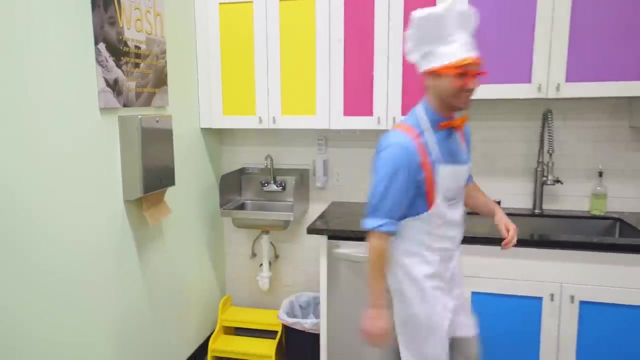 All right, there we go. Let's rinse them off. It's really important to rinse off your hands and wash them completely After touching raw eggs or meat or anything like that. Now we're ready. Okay, All right. next we're going to want to do a cup of panko, Okay. 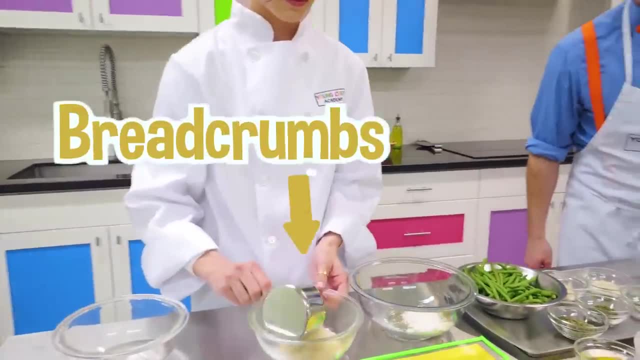 That looks about right. Yeah, So is panko. just like breadcrumbs, It is. It's dried breadcrumbs. Okay, All right, I'm going to just use that. Okay, All right. Oh, I'm going to just use that. 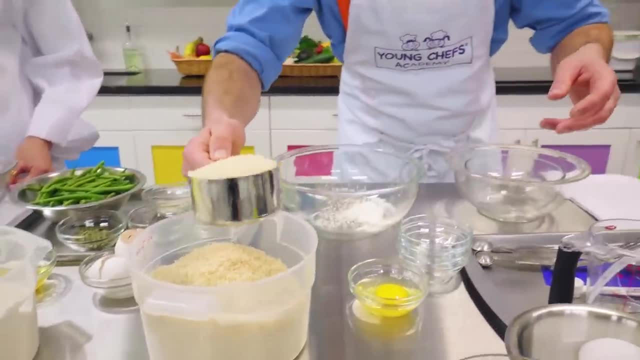 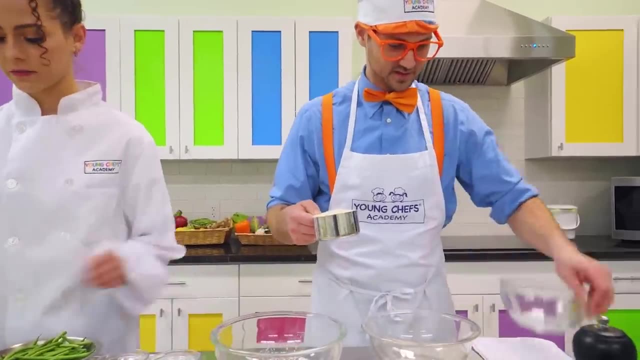 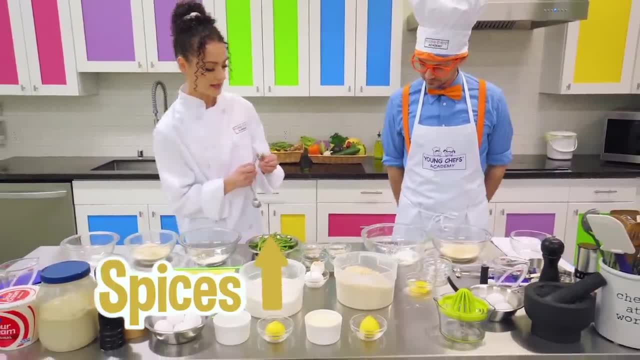 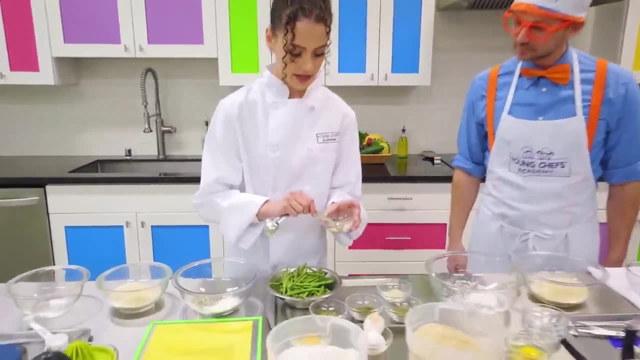 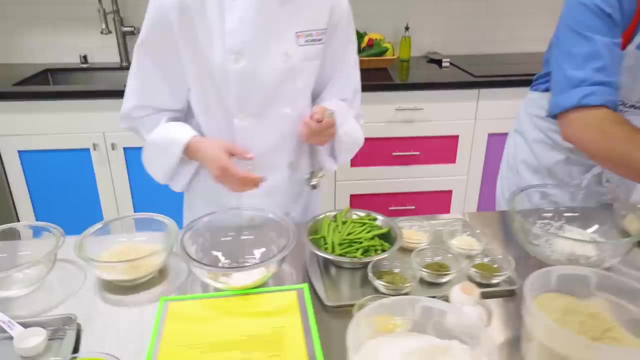 All right. Next, we're going to want to add the rest of our spices, which is garlic salt and salt. Okay, So we're going to want to use a a fourth of a teaspoon of garlic salt In our panko. Okay, Here we go. 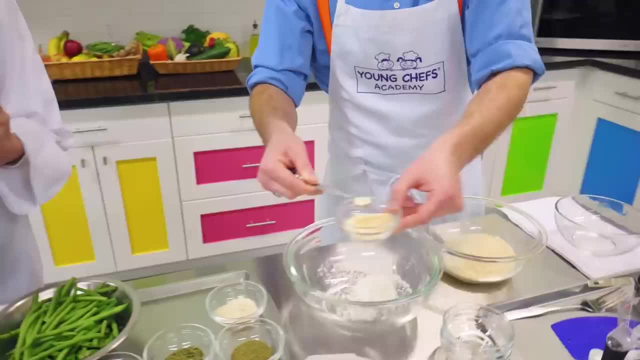 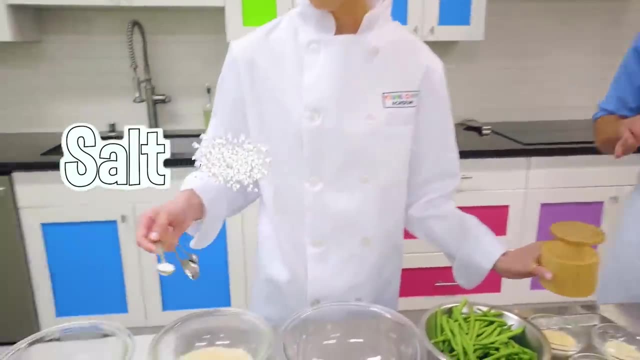 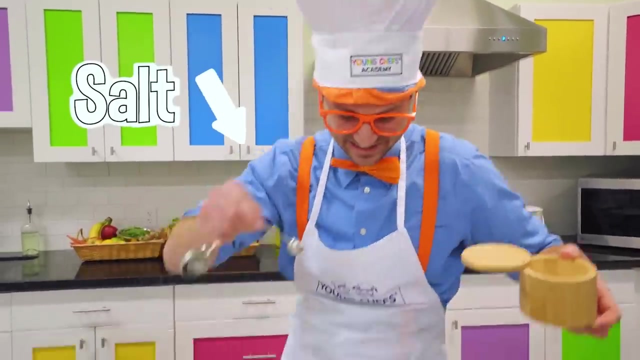 This one, Mm-hmm, Okay. And then put it in the panko: Perfect. And then half of a teaspoon of salt, Okay, Thank you. Wow, Salt is so yummy, Here we go. Can you use your whisk and whisk that up? 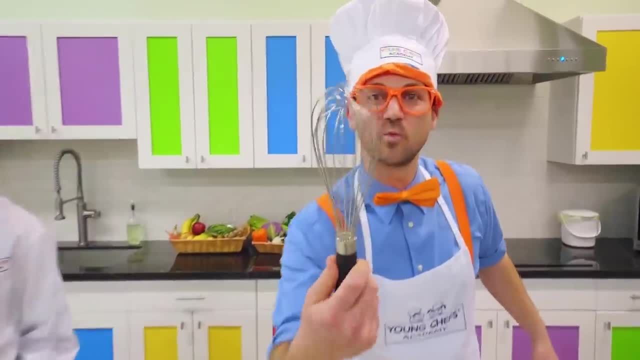 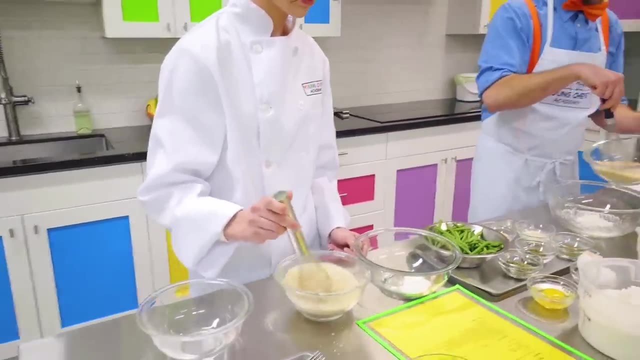 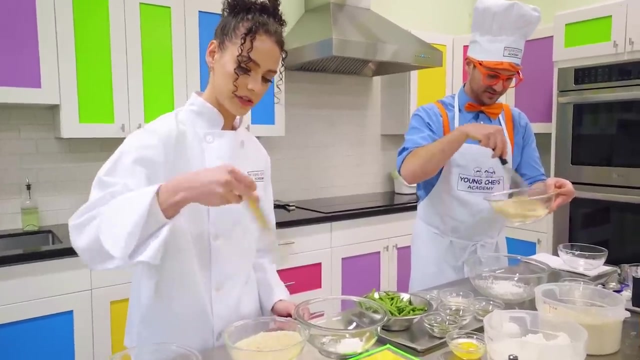 Yeah, Oh, chicken, Check it out. This is a whisk. Yeah, How do you do it? Whisk with your wrist. Okay, Whoa, This is a really good way to mix it all up. Good job, Yep, You want to use it like that. 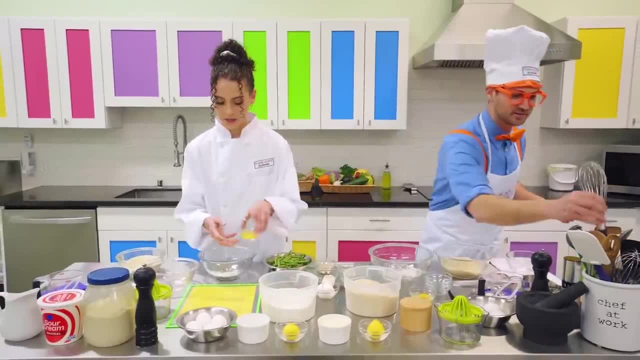 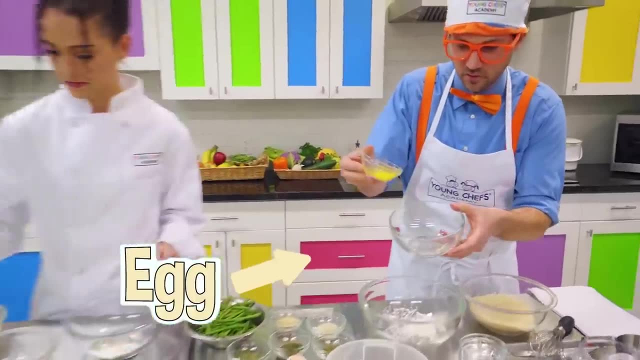 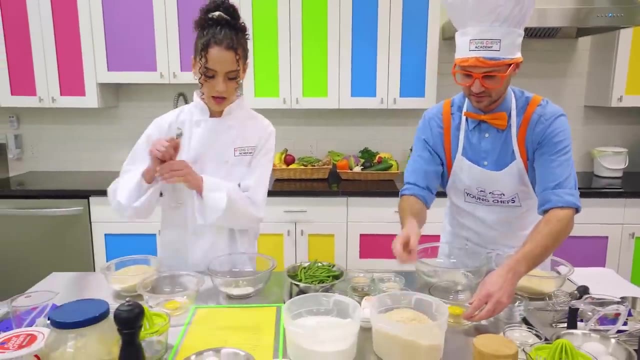 All right. Next, we're going to want to put our egg into this mixing bowl, The clean mixing bowl that we have. Okay, There we go, Put the egg in this bowl. Wee, Oh, All right. And we're going to want to use a little bit of water. 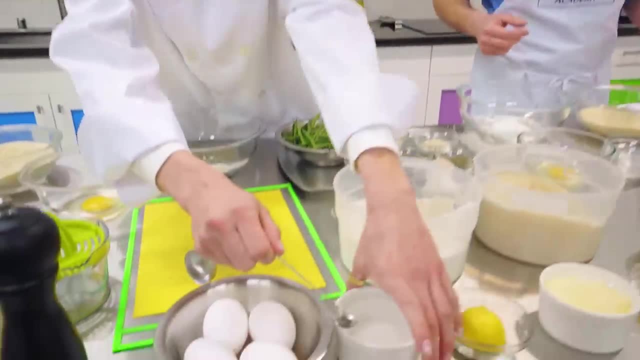 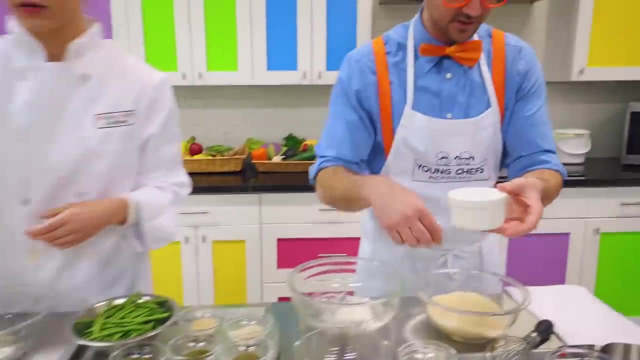 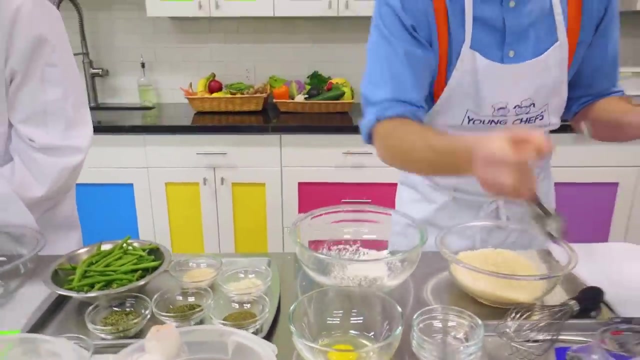 A little bit of water like this In with the egg Perfect. Thank you All. right, Put some water in with the egg Perfect. Can you whisk that? Whisk that egg up with the fork, for me With the fork. 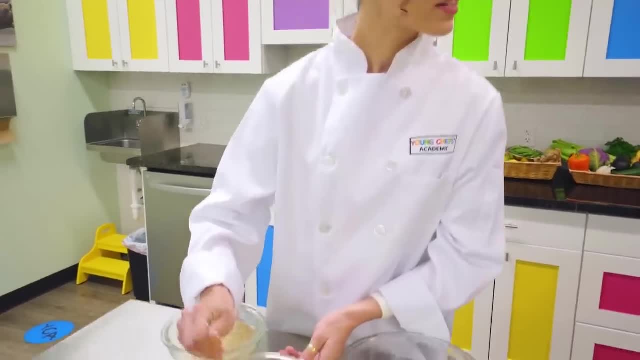 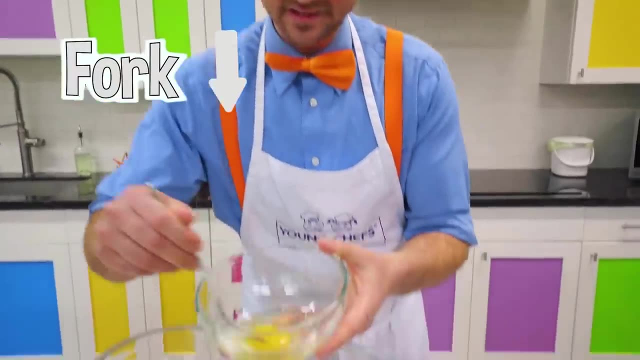 Okay, Forks are easier to whisk eggs than a whisk is. Oh, So you want to whisk it, just like that? Okay, So let's take the fork and let's whisk the egg. Whoa, Did you see how the yolk broke up? 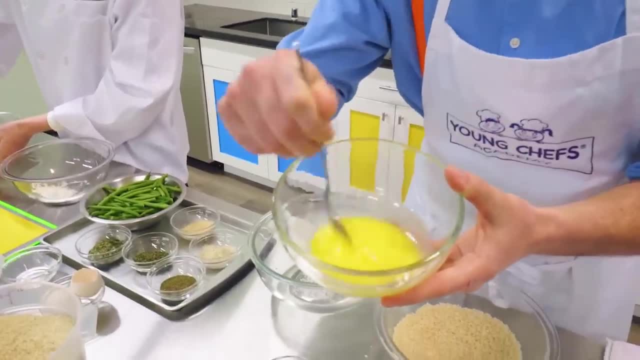 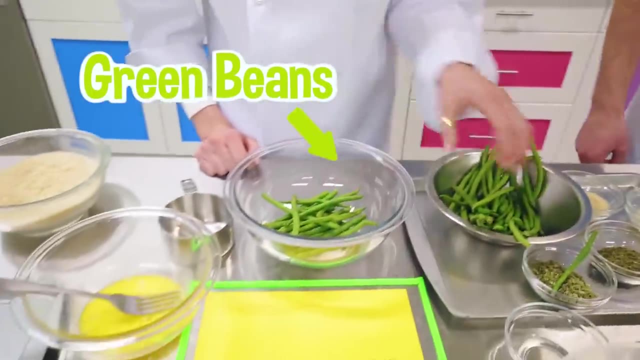 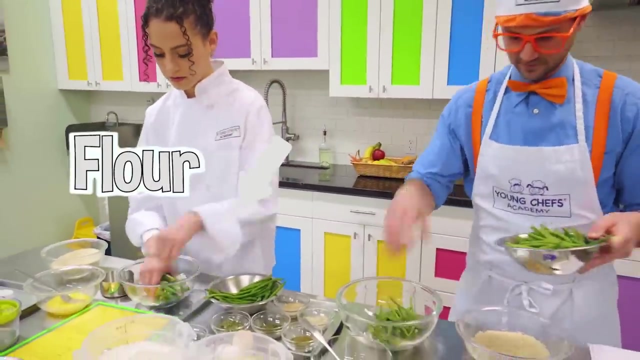 And now it's all mixed up, Perfect, Perfect. We're going to grab a couple of hands. We're going to grab a handful of green beans right in here. Okay, All right, Perfect, And toss it in our flour, All right. 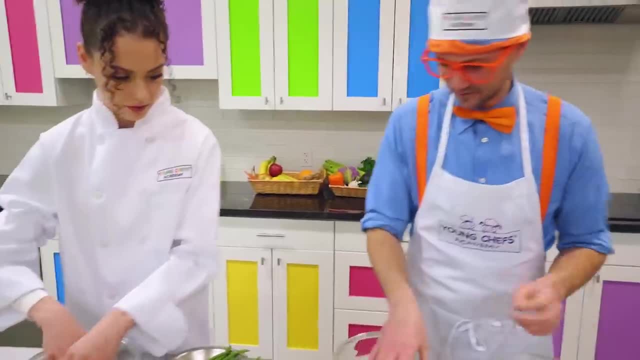 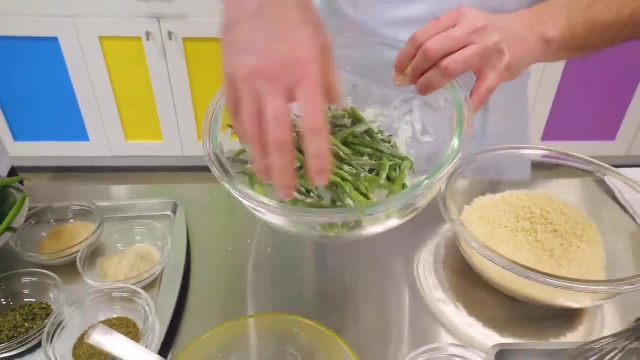 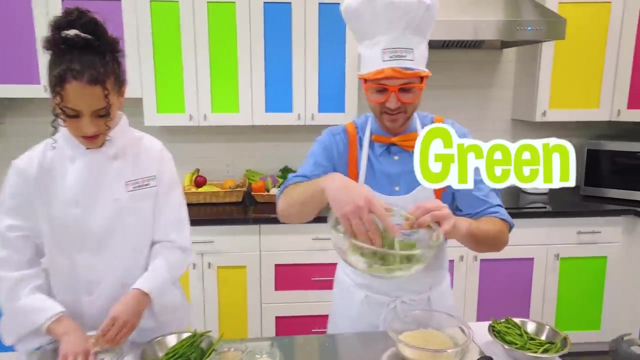 Make sure you get them all nice and mixed up and coated in flour. Okay, Toss it. Wow, This is going to help the egg stick to the green bean. Okay, Interesting, Look, They used to be green, But now they're green. 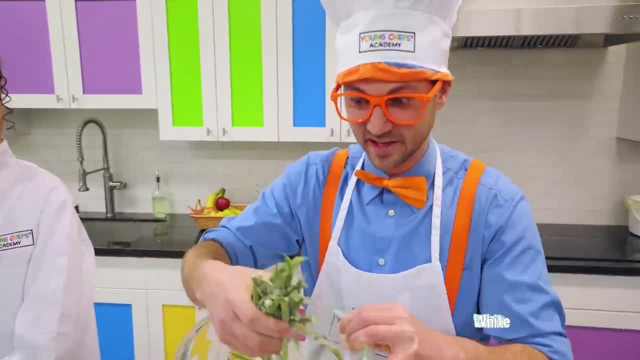 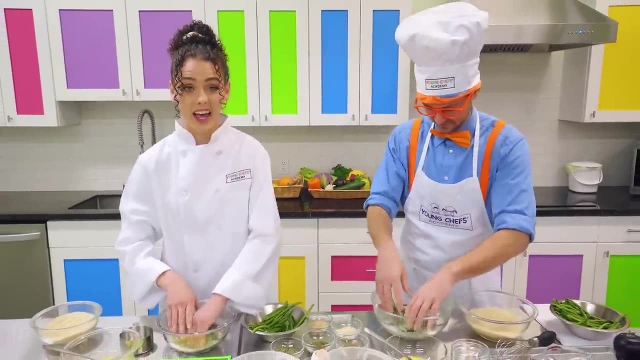 And white. Hey, remember how we washed our hands? Yeah, Good thing we did, because I'm touching food with my hands. You don't want to touch anything after you touch egg or raw meat. You want to make sure you wash your hands. 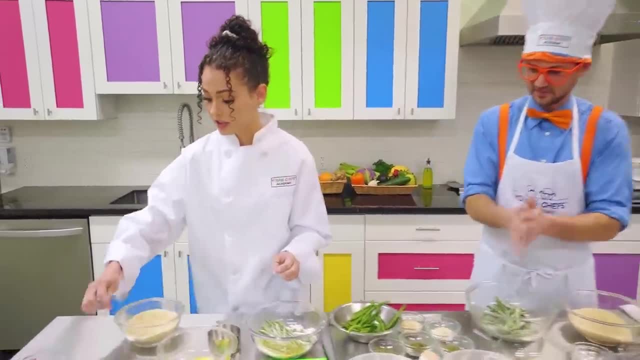 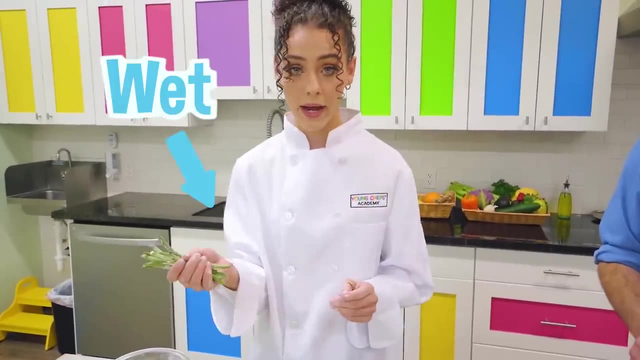 Okay, All right. Now we are going to touch the egg, We're going to put the green beans, We're going to use two different hands. We're going to have our dry hand and our wet hand, So we're not going to touch the egg with this hand. 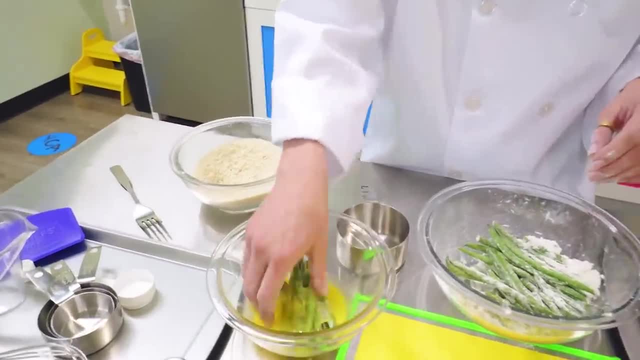 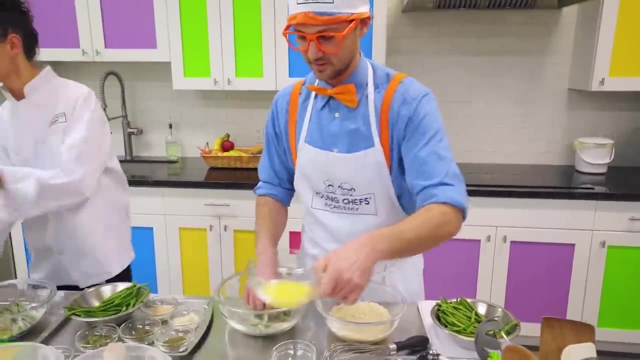 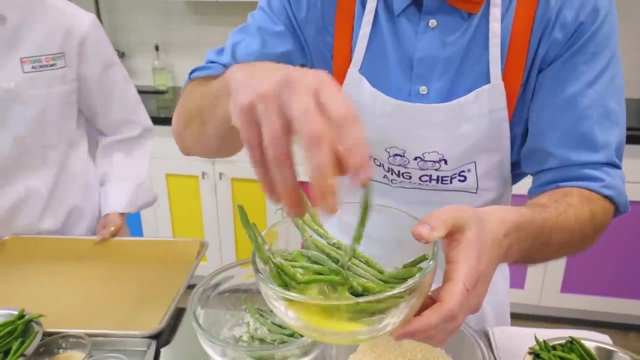 We're going to put our green beans in here And toss it around. Okay, Take the fork out Now do a little tossing, There we go. Whoa, I'm spilling, That's okay. Okay, Wow, Look at it. 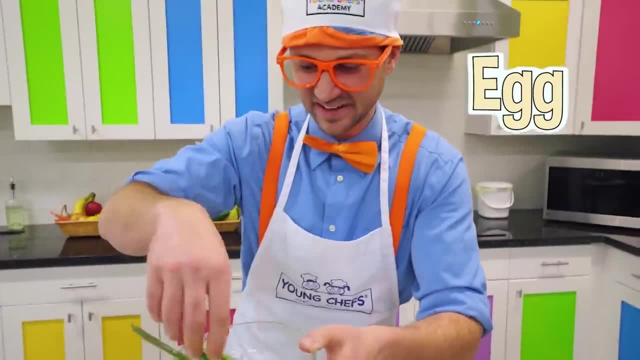 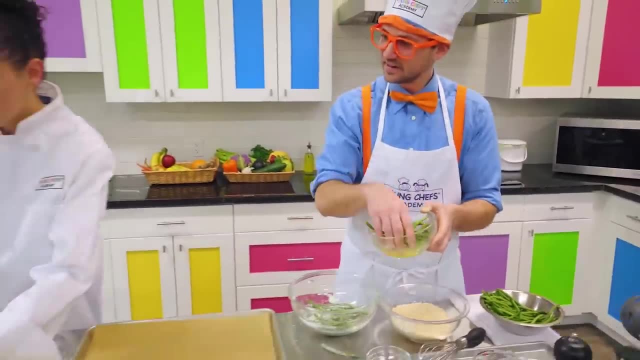 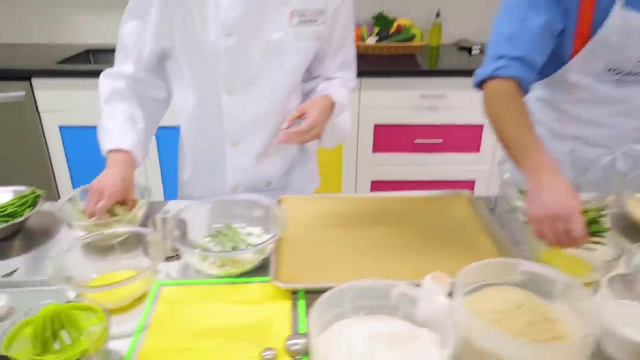 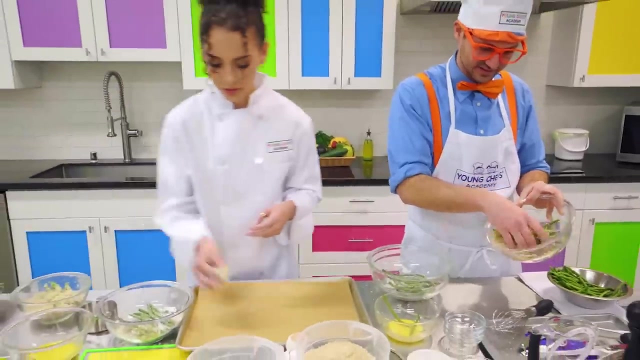 There's so much egg on these green beans? Okay, All right, Great. Now you're going to want to put the green beans into the panko. Toss them around real quick. Okay, Wow, That looks fun. And once they're nice and evenly coated in panko, you want to put them onto the tray. 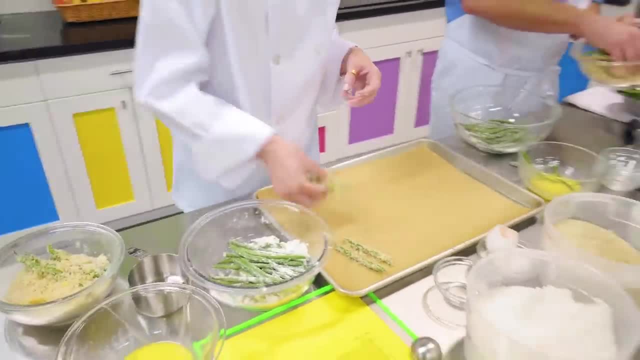 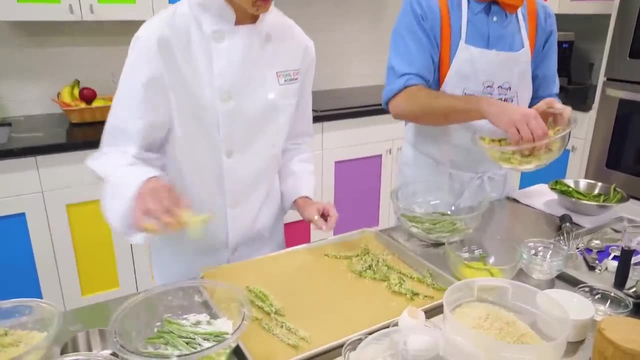 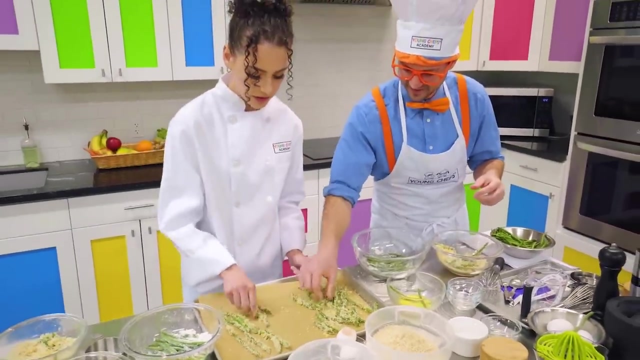 Okay, Whoa, These are going to be so yummy. I know I'm excited. Let's put them a little bit nicer so that they're not so messy. Okay, That way they'll cook really evenly when they're spread out on the tray. 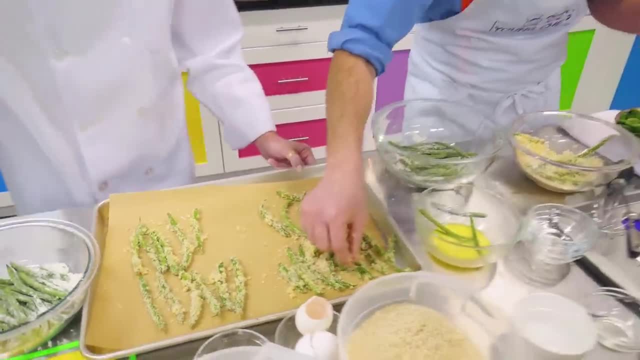 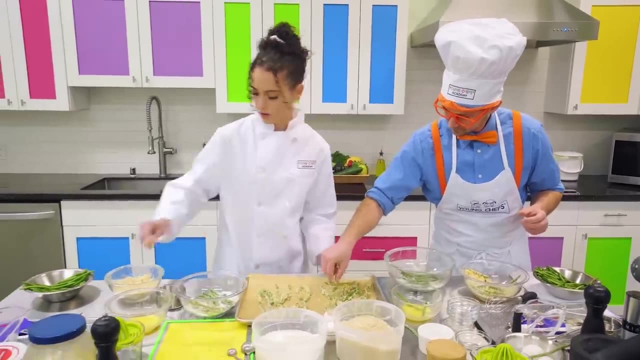 There we go. That makes sense. Oh, I see, Because if they're on top of each other then the heat can't touch the whole green bean. huh, Exactly, You want to make sure that the whole thing is getting cooked. 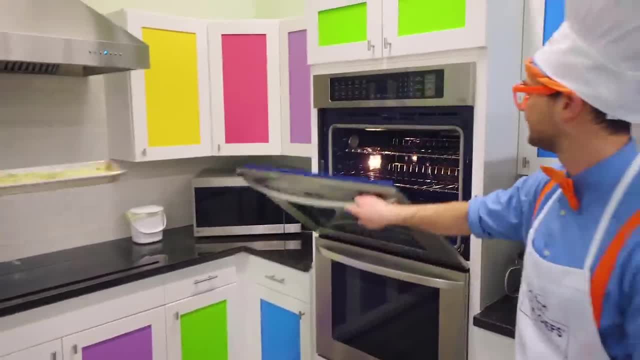 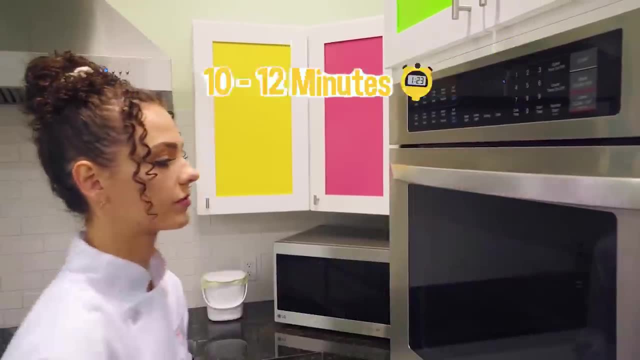 We're ready for the oven. Okay, There you go, There you go. Thank you, Perfect. Those will take about 10 seconds, 10 to 12 minutes to cook Whoa. That was really fun making those green beans with you. 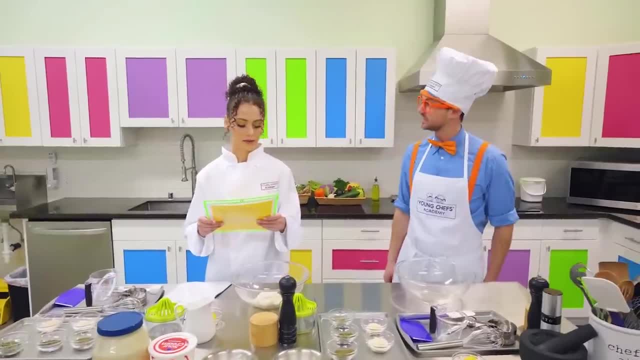 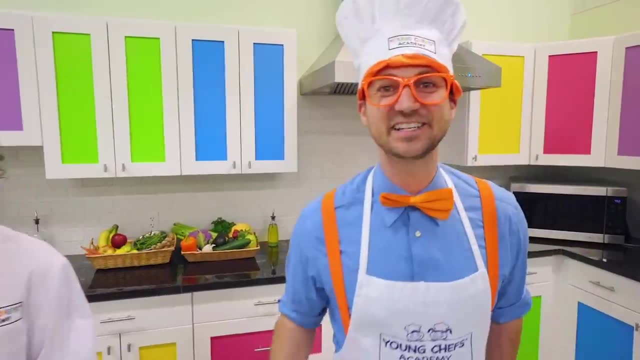 Wasn't it? Yeah, Let's make some ranch to dip them in. What ingredients do we need? We need mayonnaise, sour cream, buttermilk. Oh wait, Did you say buttermilk? Yeah, Oh, I said cream earlier. 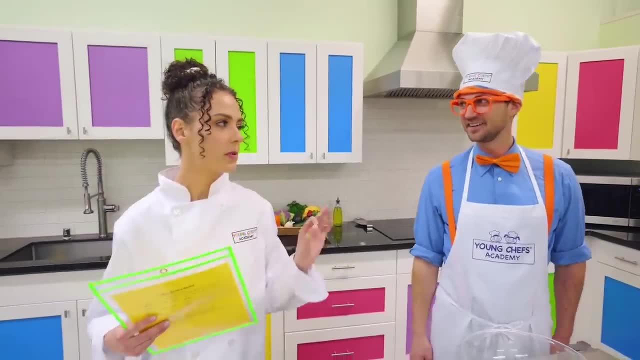 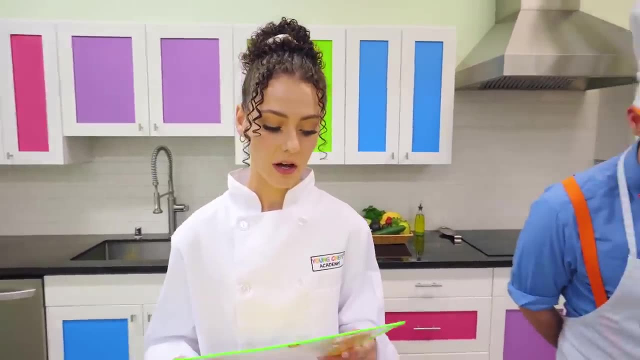 Okay, So we need buttermilk. Yes, They're very similar, but buttermilk smells different and it's a little thicker. Okay, All right. Lemon juice, dill, weed, parsley, chives, onion powder, garlic. 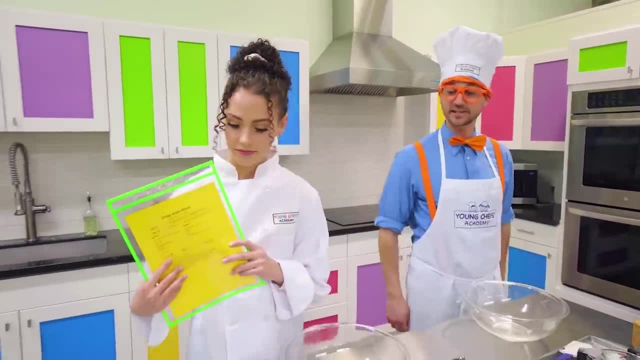 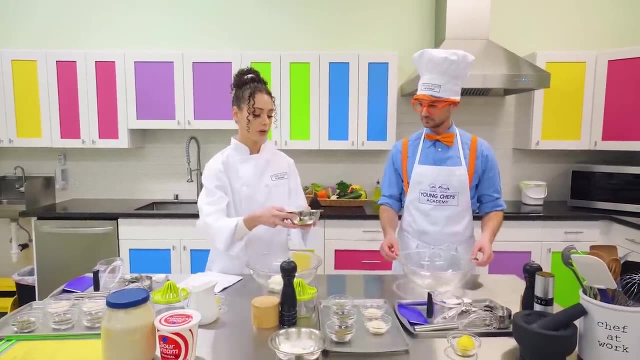 Garlic powder, salt and black pepper. Okay, Perfect, Looks like we have everything I think we do. All right, Next we're going to want to, So I have mine all mixed up. Can you put the mayo and the sour cream into your big bowl? 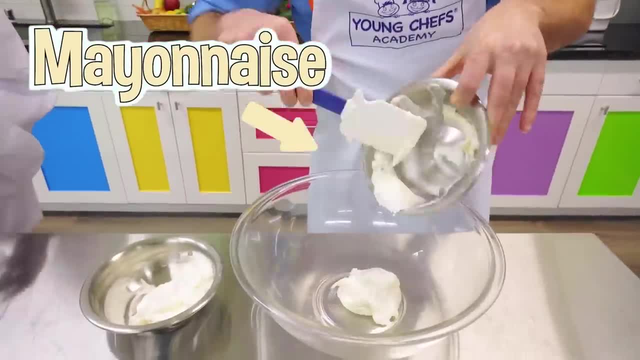 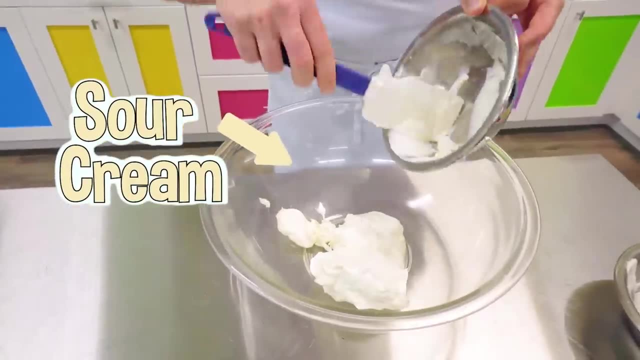 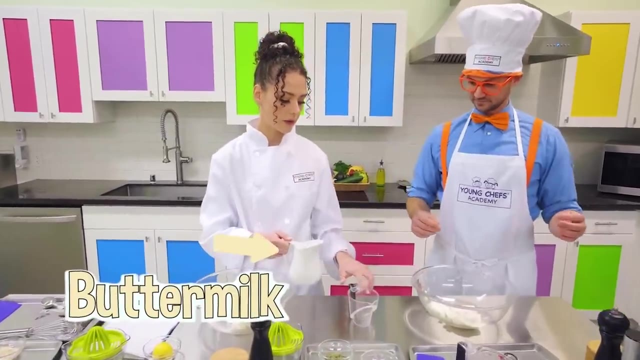 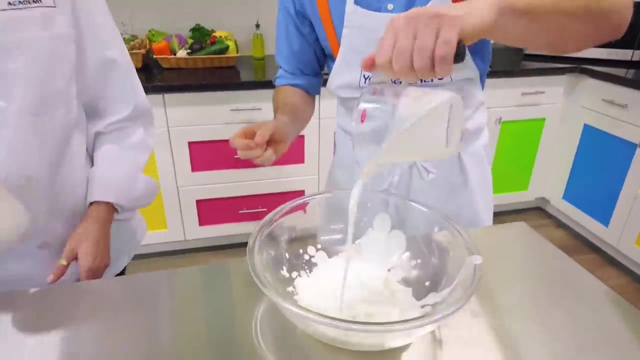 Okay, Here's the mayo. Then we have the sour cream. All right, There we go. Awesome, Now we're going to want to do half a cup of buttermilk into your bowl. Okay, All righty, There we go. 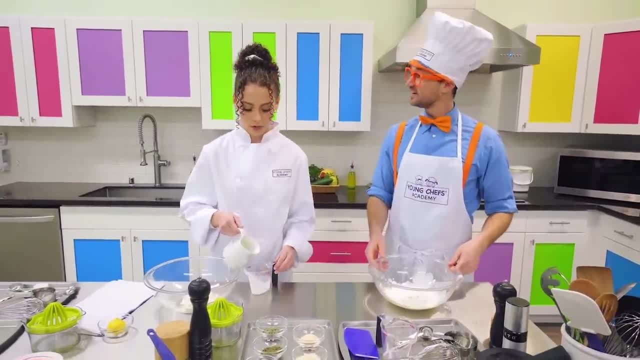 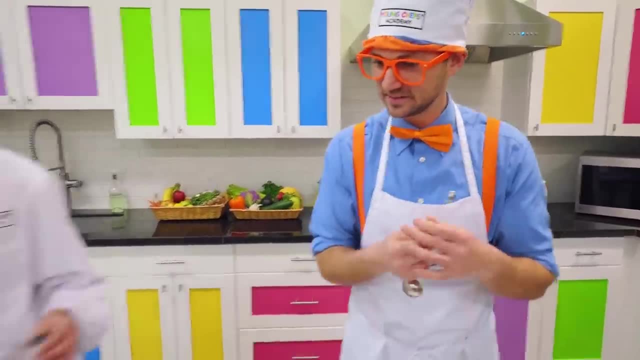 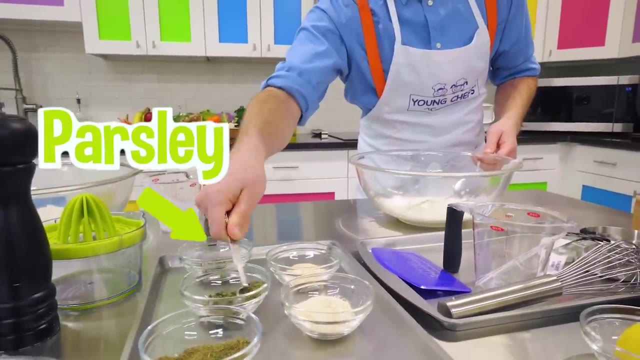 Perfect, All right. Now we're going to want to get our one-fourth teaspoon. Okay, Perfect, I'm ready, And we're going to use that for our dill right here: parsley and our chives. Okay Dill, parsley and chives. 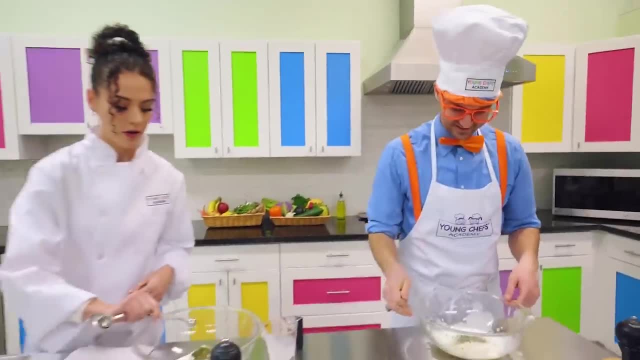 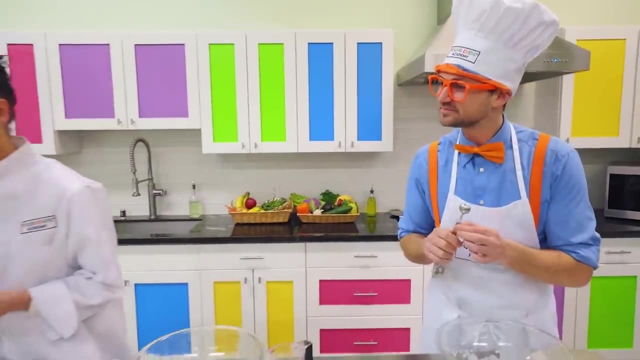 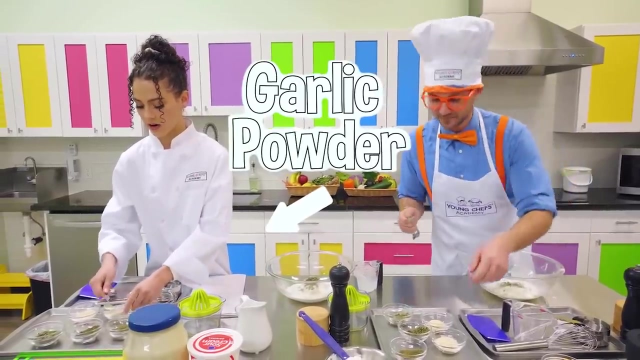 There we go. Good job, puppy. Next we're going to want our half teaspoon- Okay, A little bigger, All right. All right, And we use that for our garlic powder and our onion powder, All right? Okay, Let's give it a little scoop. 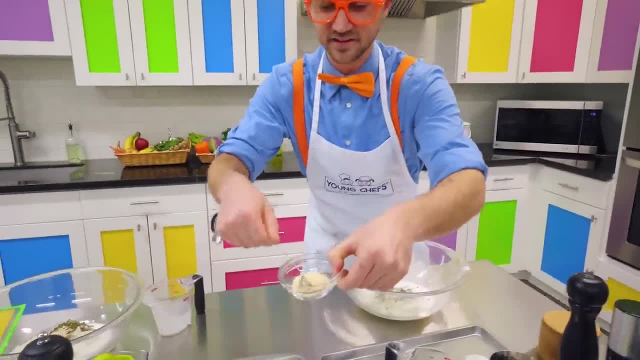 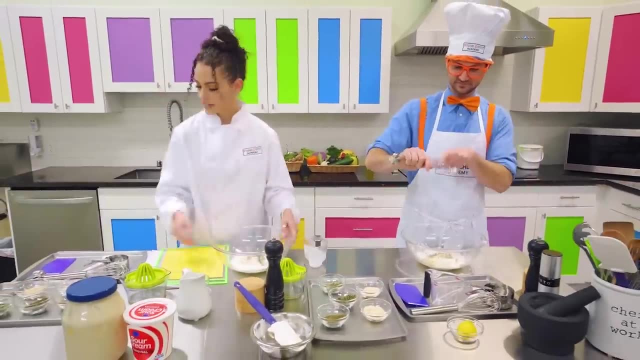 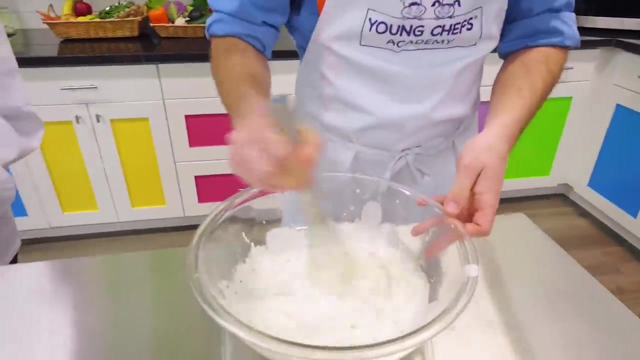 Okay, And then this one. Perfect. This is going to be so yummy. All right, Perfect. Let's mix that up with our whisk. Don't forget, we whisk with our whisk. All right, Whoa, This smells so good. 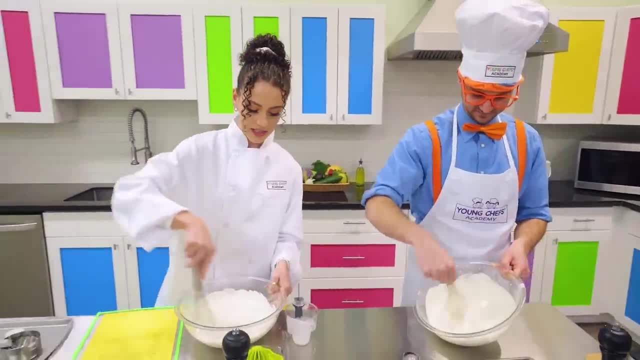 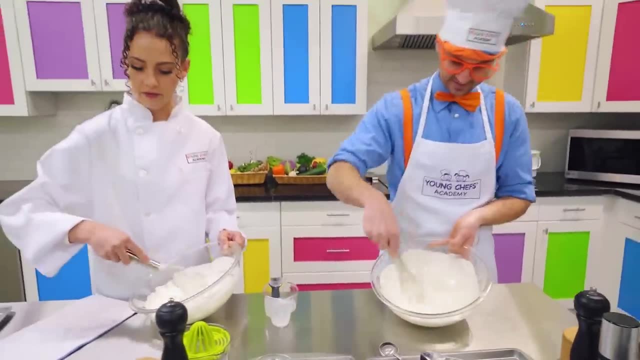 Once it's all mixed up, we're going to cover it and place it in the fridge. It's going to cool. All right, We only have three more ingredients. Okay, What are they? Lemon juice, salt and pepper. Okay. 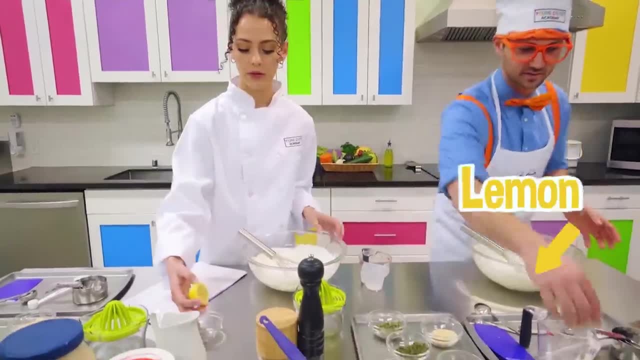 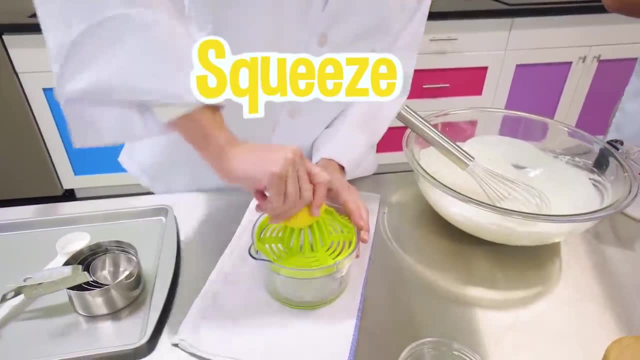 First, we want to juice our lemon. Okay, So you have a lemon right up there, Perfect, We have it cut in half and we'll use our juicer here. We want to make sure we squeeze really tight, pushing down and twisting it around to get. 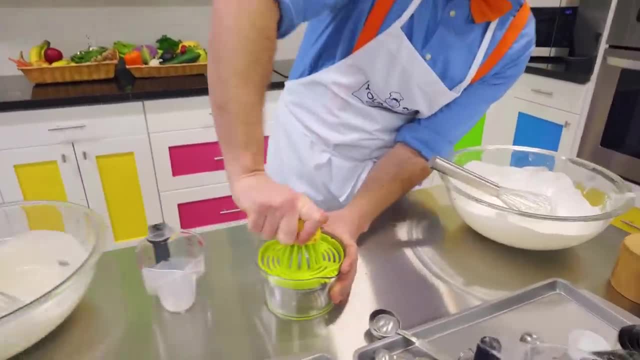 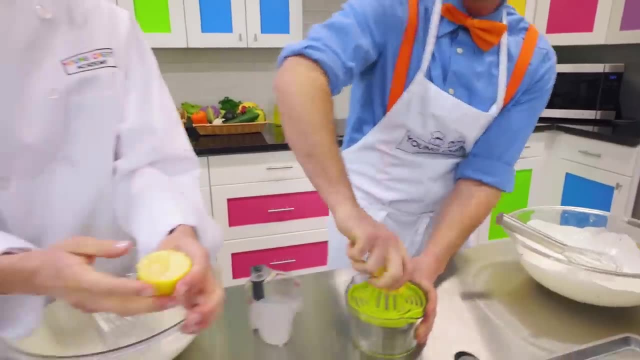 all of that juice out. Okay, I guess I'll try it. Oh, There we go. Good job, Yeah. When you take it off, your lemon should look something like this: Yeah, It's almost empty. Perfect, Good job. 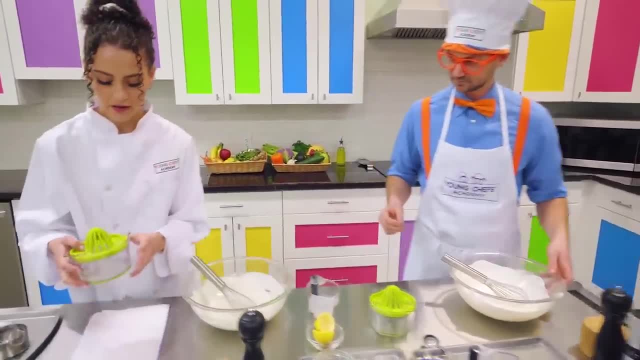 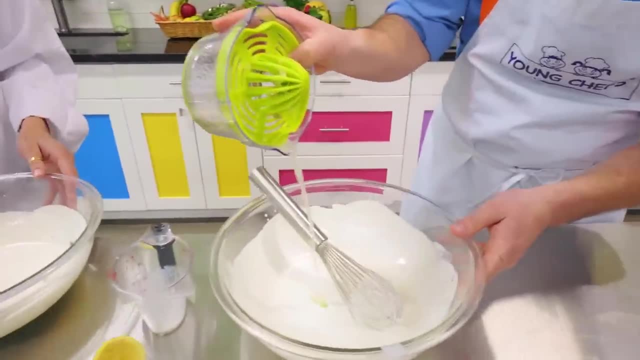 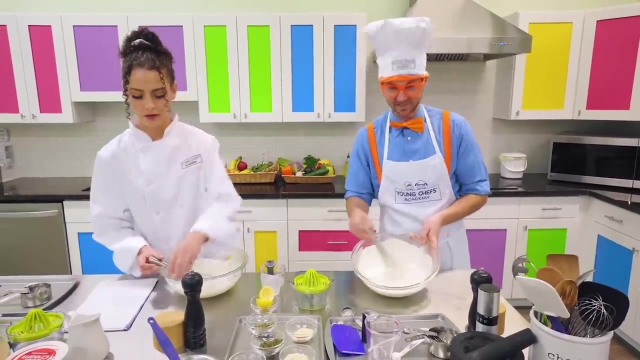 Okay, Put this down for you, And then we'll want to pour our lemon juice into our ranch. Okay, Here we go. Whee, Awesome, Mix that up. All right. Now we want to do one-fourth teaspoon of salt. 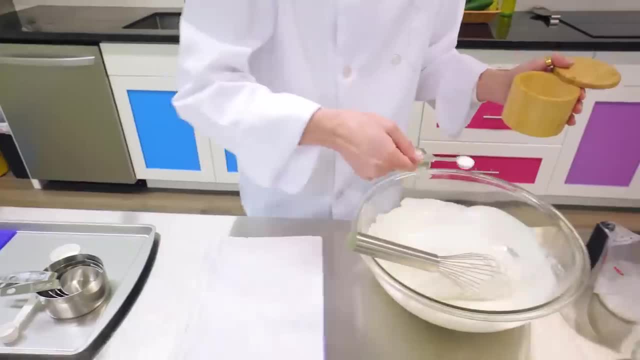 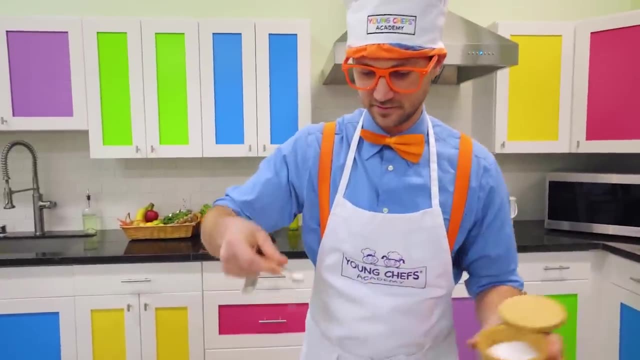 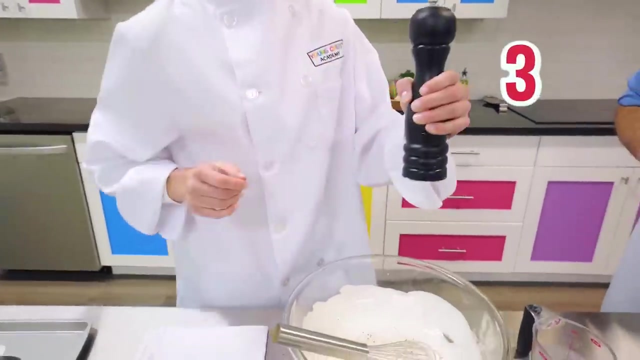 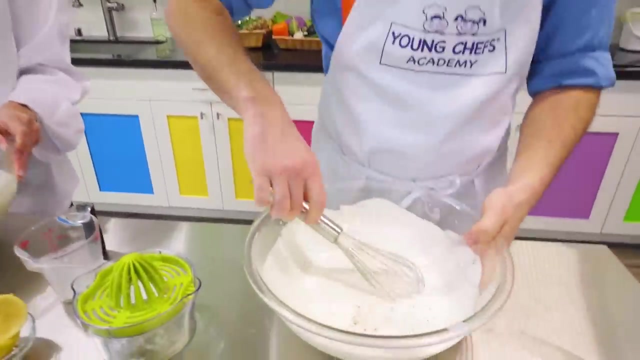 Right like this: Okay, Put some salt in here. There we go, Whee And a pinch of pepper. So we'll go about three twists. Okay, One, two, three, Perfect. All right, Let's mix that up. 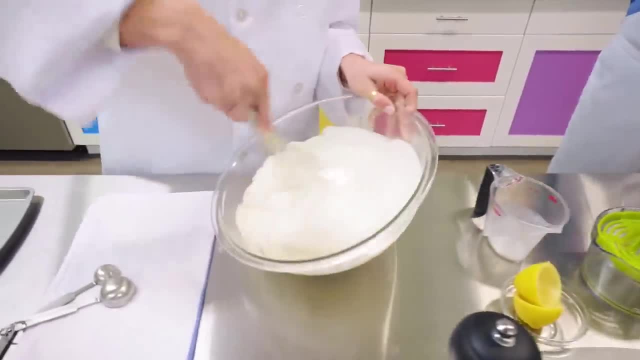 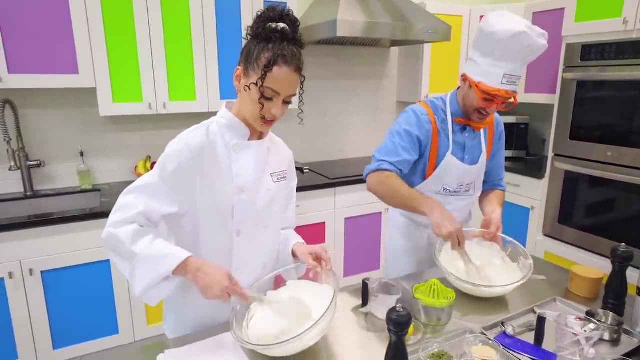 All right, Mix, mix, mix. Remember to mix with your wrist. Oh yep, Oh wow. This is going to be so yummy, It's going to be delicious. Did you hear that? I did. Does that mean the green beans are done? 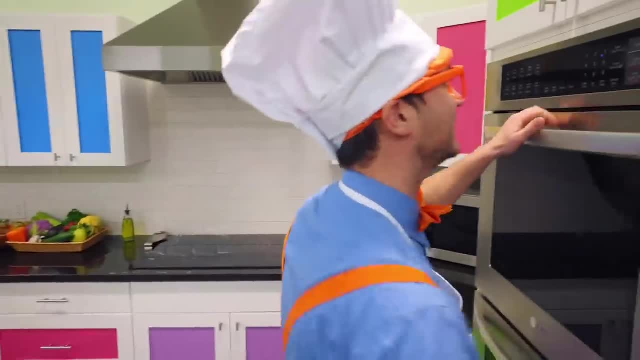 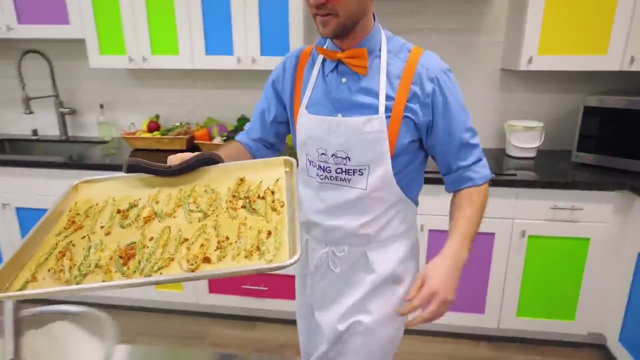 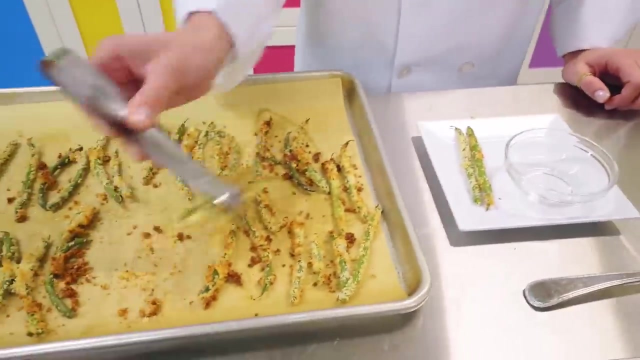 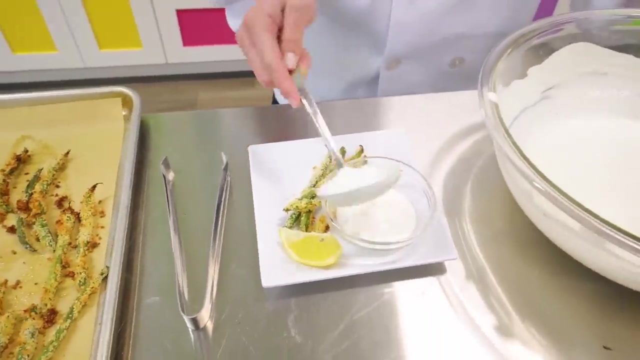 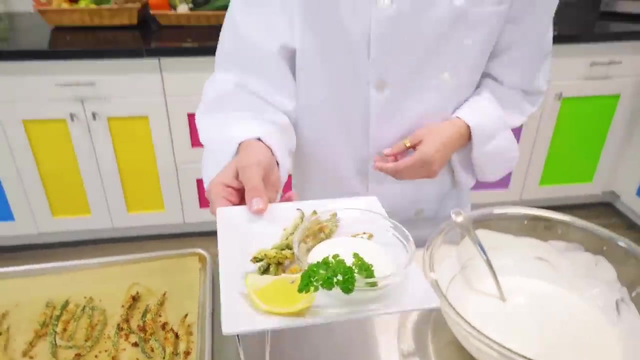 It does. You want to grab them? Sure, Oh, this is going to be awesome. Oh, yum Wow, Those look delicious. Blippi, Whoa, Check them out. Oh my gosh, All right, Blippi. 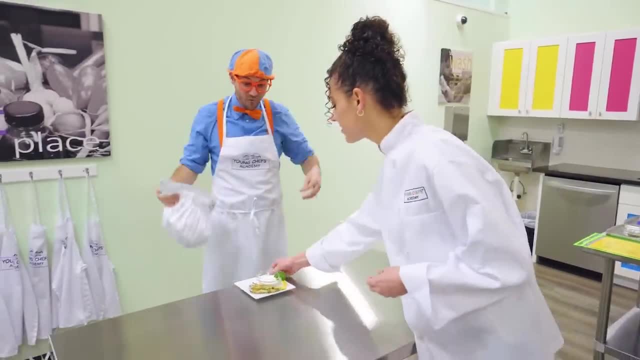 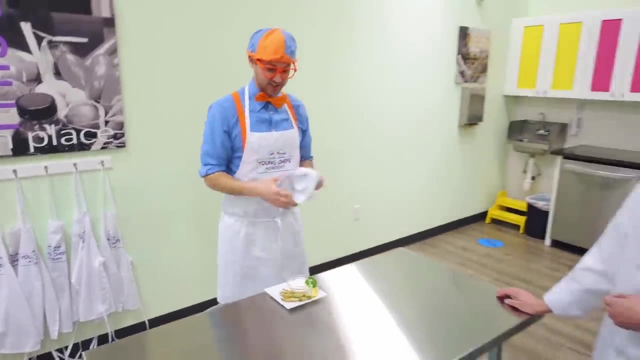 It looks like our green beans and zesty ranch are all ready. They look so good. Those look yummy. Check them out. Whoa, I am so excited. Thank you so much for teaching us how to make these. Of course, You did such a good job.